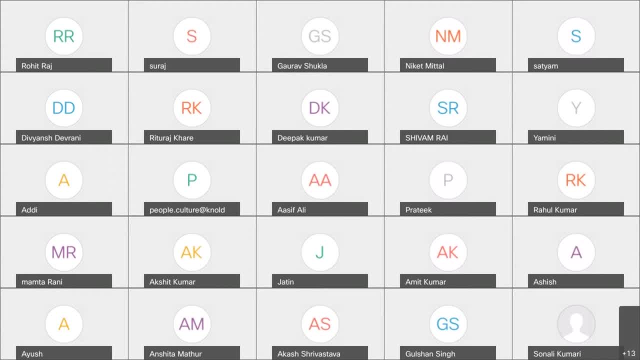 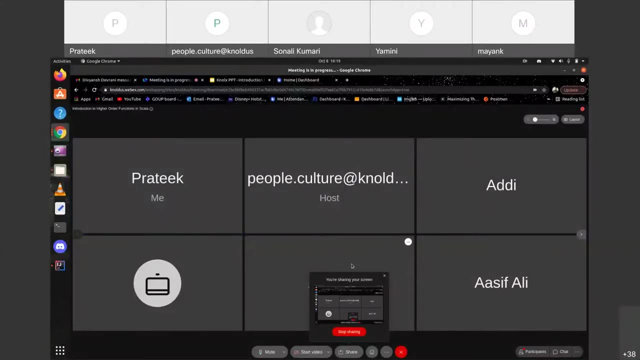 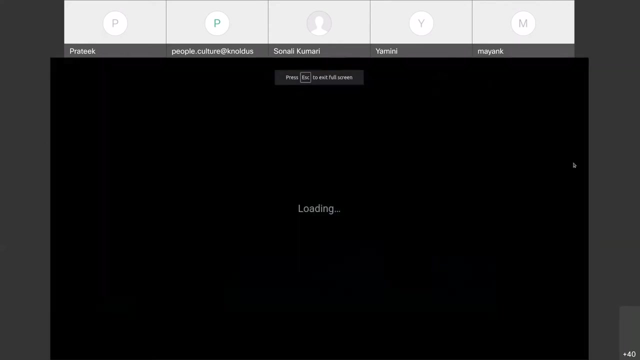 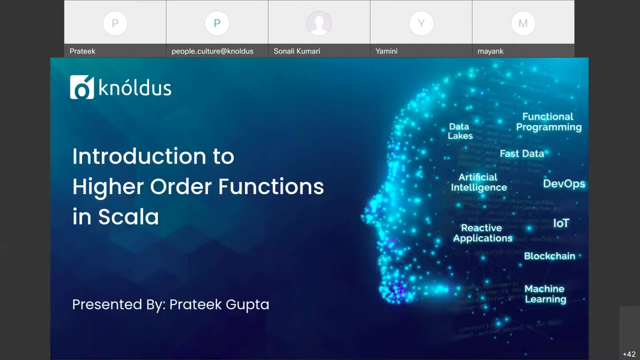 a good attendance of that. Okay, sure, Let me see the screen first. Okay, So is my screen visible to everyone? Yes, Prateek, Okay. So, Gurpreet, can we start now? Hello, Yes, Prateek, we can start. 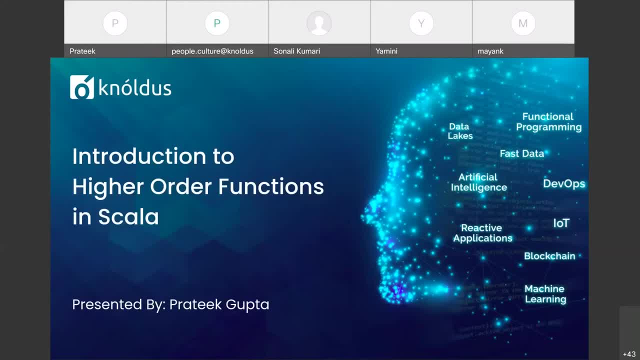 Okay, thank you. So hi everyone. First of all, welcome to this knowledge session. My name is Prateek Gupta. I'm a software consultant at Naldus, So in this session I'll give you a brief introduction for high order function in Scala. 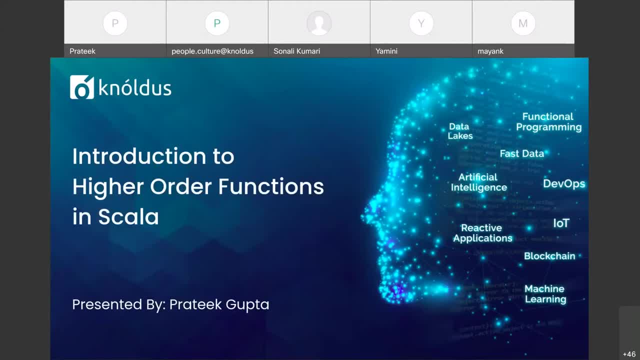 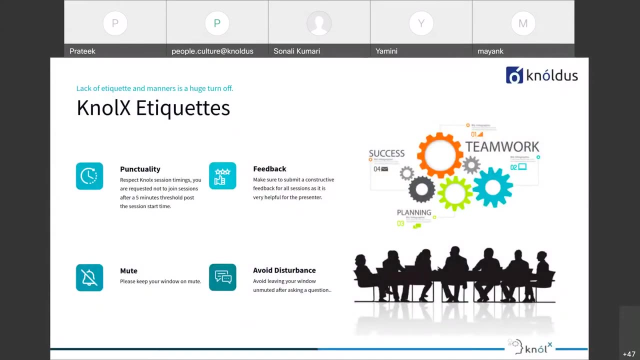 So hopefully it's going to be an easy session for everyone and also a quick one. So before beginning, let's quickly discuss about the knowledge etiquette. So first one is punctuality. So it is always recommended for everyone to join the session at least five minutes before. 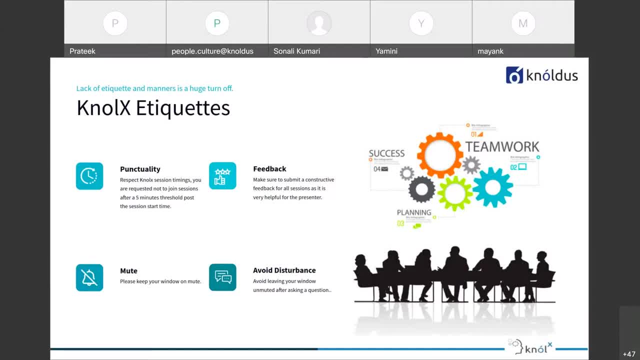 it gets started, so that we can start the session on time. Next one is mute. So please keep your window on mute until you have any question. So if you have any question, you can unmute yourself anytime. Next one is punctuality. 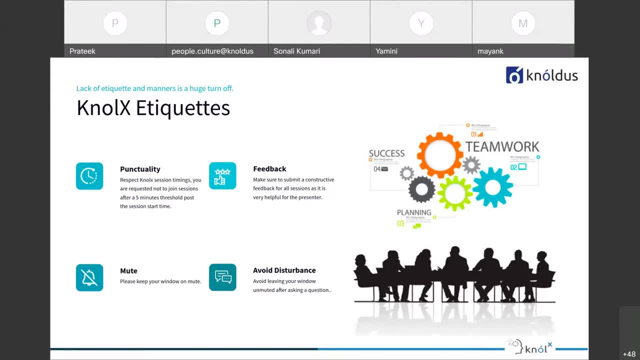 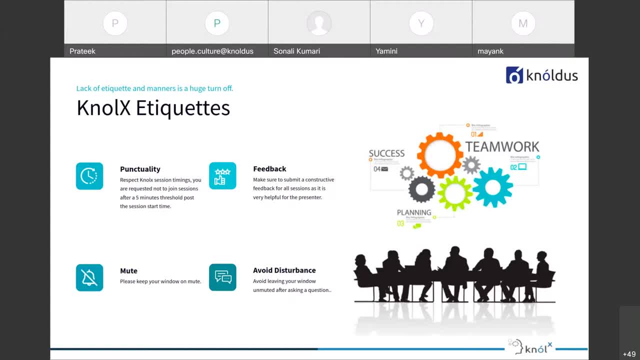 And the final one is feedback. So make sure you submit the feedback after every session, because it is really helpful for the presenter to present you more better next time. So Now let's move on towards the agenda for today. So am I audible now? 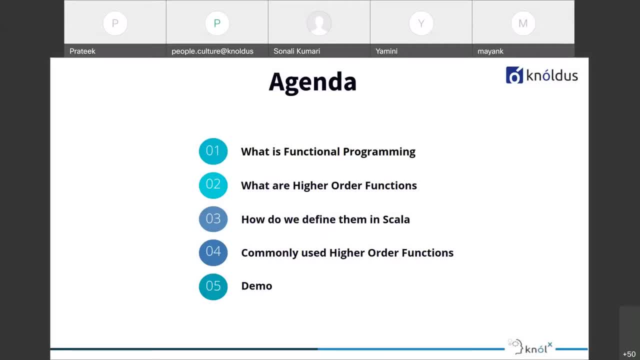 Yes, So our agenda for this session will be: first, we'll go through what is functional programming, as it is a base to understand what are high order functions. Next we'll move on to the high order functions. what are they? Then we'll see how we can define them in Scala. 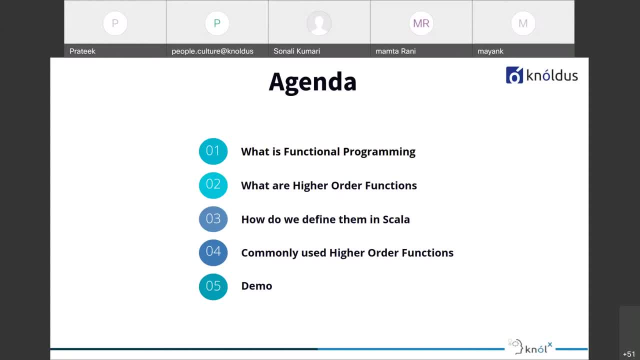 And after that we'll learn about some of the commonly used high order functions in Scala And finally, a demo where we'll try to see some example. We'll see some example of high order functions, how we can define them in Scala. 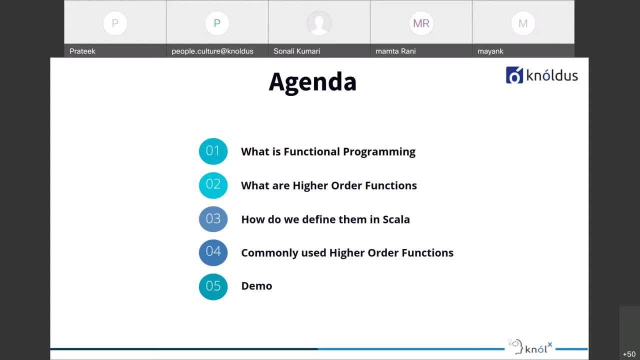 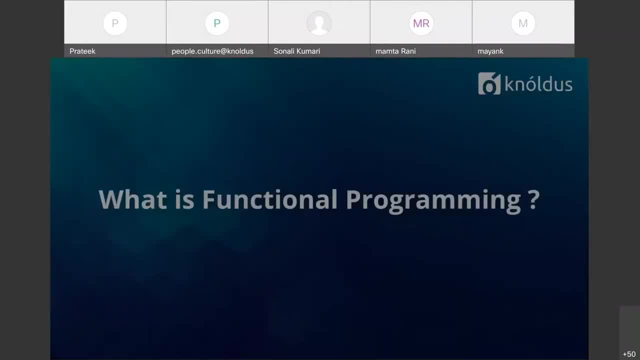 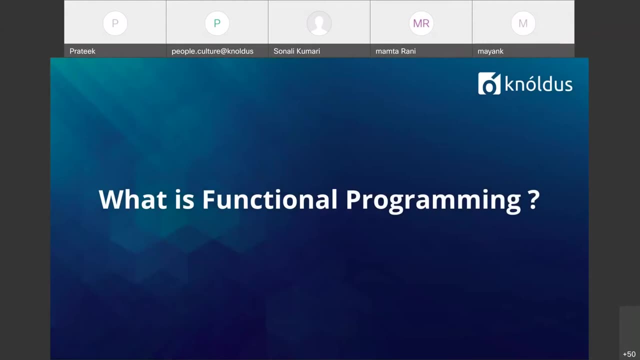 And we'll also use Scala And some of the predefined high order functions in that demo part. So let's begin. So, apart from being a purely object-oriented programming language, Scala is also functional, So we need to understand what is functional programming. 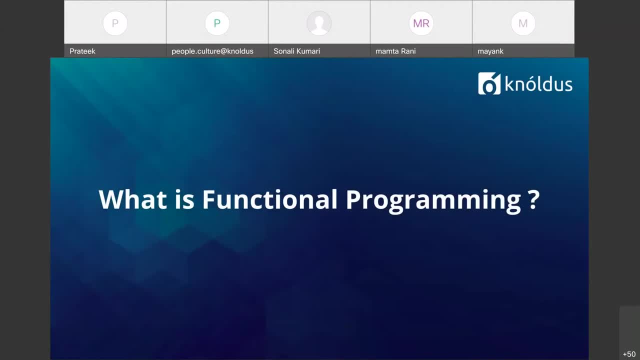 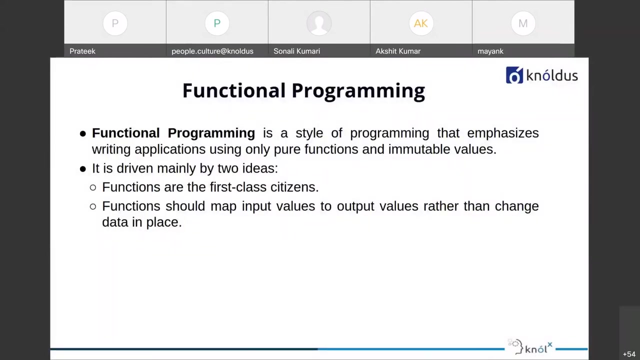 So anybody who would like to answer this question, Anyone. Now, it is a way to write programs that create eigenmathematical functions. Okay, Right, Anyone else Okay. So let's understand a bit more about it. So functional programming is basically a style. 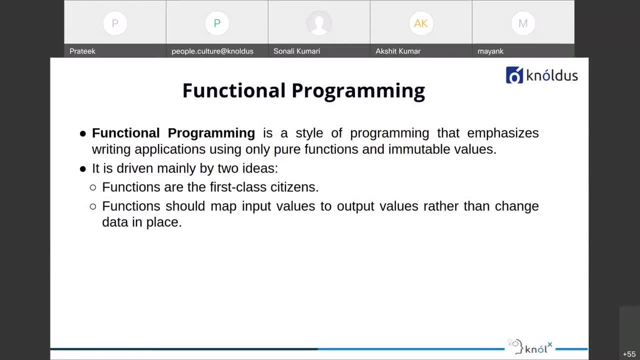 It is a style of programming that emphasizes writing applications using only pure functions and immutable values. So pure functions in the sense that those functions that does not have any side effects. So what are side effects? So a function is said to have side effects if it does something other than simply returning a result. 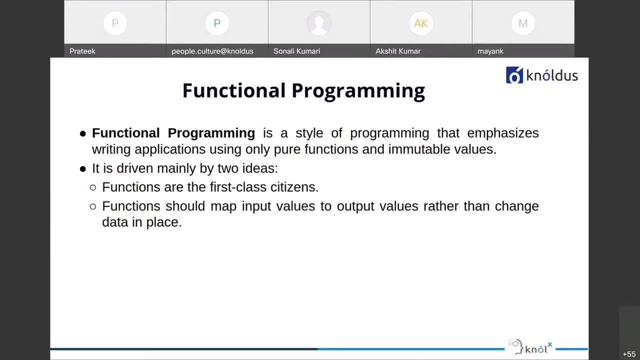 So, for example, modifying a field or printing a file. So, for example, modifying a file or printing a file. So, for example, modifying a file or printing a file, That says part of the case that this object is getting to the console. 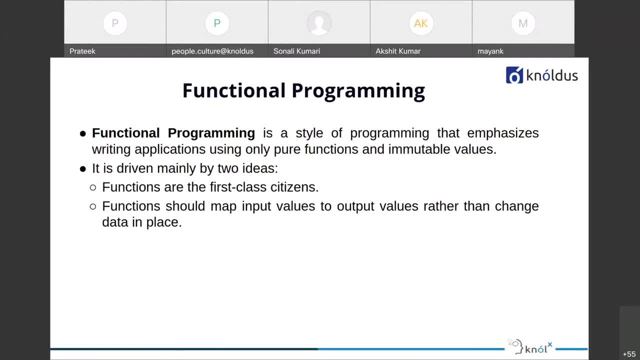 reading input from the console, reading from a file or writing from a file and such kind of things. That's not cup and cup but actually a microcon backdrop, Да, And such kind of things. Okay, So functional programming works well with immutable values. 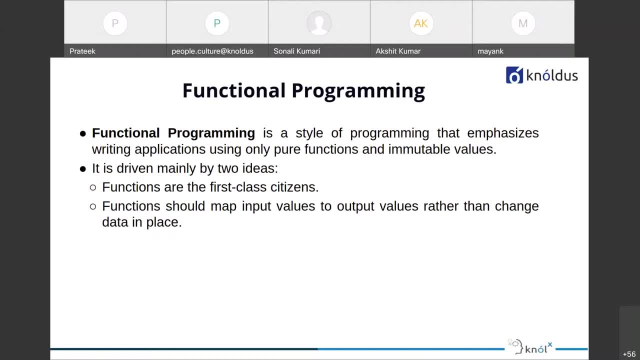 So functional programming works well with immutable values. Immutable value means something which is not changeable, Memphis. So our next point is that it is halfHow the grieving value plays a roleornally form 데 by two ideas. Of course, function programming is based, not based, on set times. Remember. So what is an impeduplace, What is a dipositive, What is an ingenuity? What is the implication of an action? What is the department filed with these which are innermate or disruption or generatorism for the? 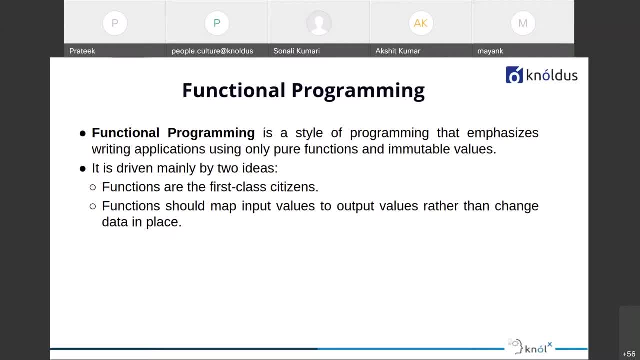 two ideas. first one is: functions are the first class citizens. so what does that mean? so functions are the first class citizens. it means that we can pass any function as an argument to some other function, we can return any function as a result to some of any other function and we can assign any function to any. 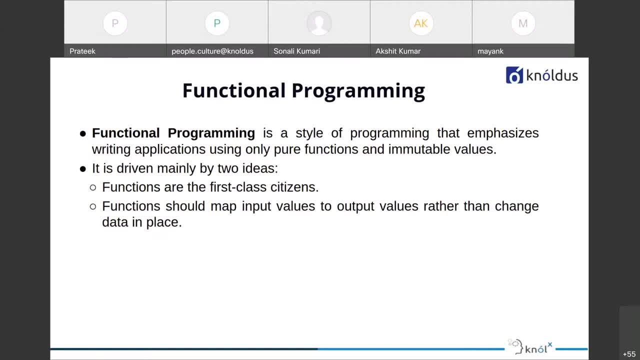 variable. so this is what first class citizens mean, like you know. you know, only in any object oriented programming language, objects are the first class citizens, so we can pass it in any function, we can return it and things like that. okay, so in Scala or in any other programming language, functions are 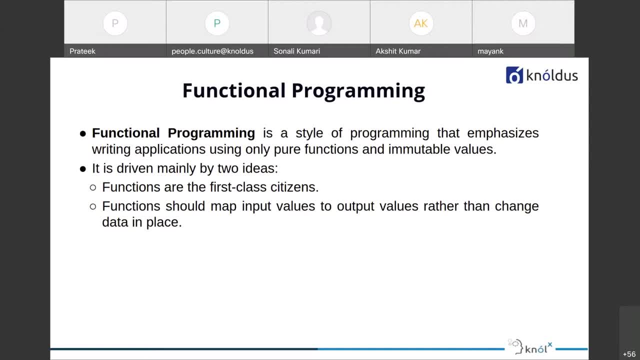 treated like any other type: string, integer or any other class type. so the next main idea is function should map input values to output values rather than changing data in place. so they help- sorry. this helps us to use the immutable data structures. so, as we have discussed ever, 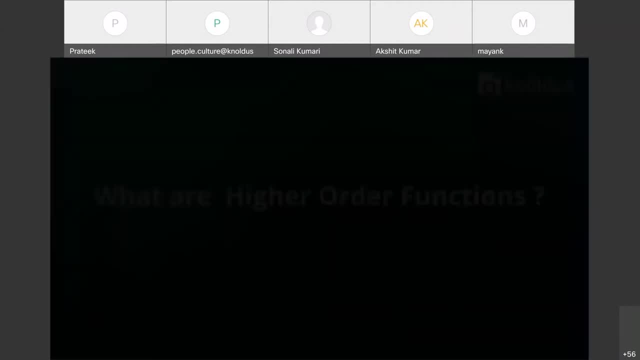 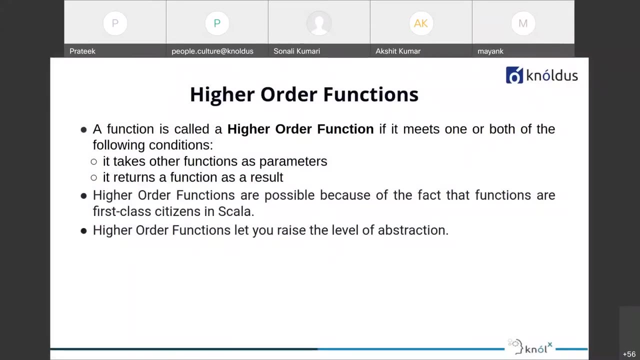 so now let's see what are high-order functions. so okay, so a function is called a higher-order function if it meets one or both of the following criteria conditions: first one is it takes other functions as parameter, or second one is it returns a function as a result. so we can say: a function is a high-order. 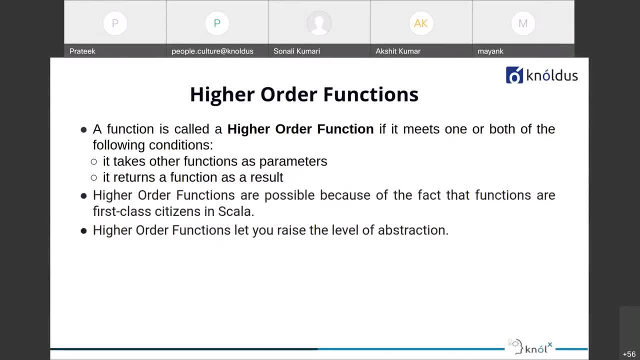 function if it can accept any other function as a argument, or it can return any function as a result, or both. it means at least one condition should met, okay. so next one is: high-order functions are possible because of the fact that functions are first class citizen Scala. so, as we have discussed in the previous, 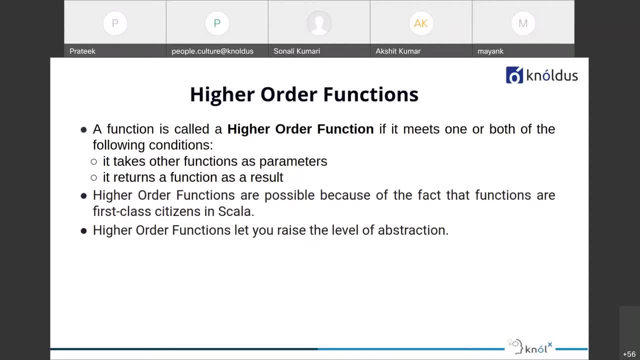 slide. functions are the first class citizens in any functional programming, and this is because higher order functions are possible. okay, so next is higher order function. let you raise the level of abstraction. so it means that you don't have to specify how things should be done, you just need to specify. 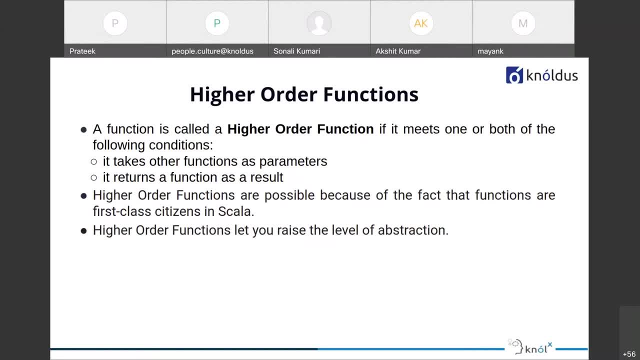 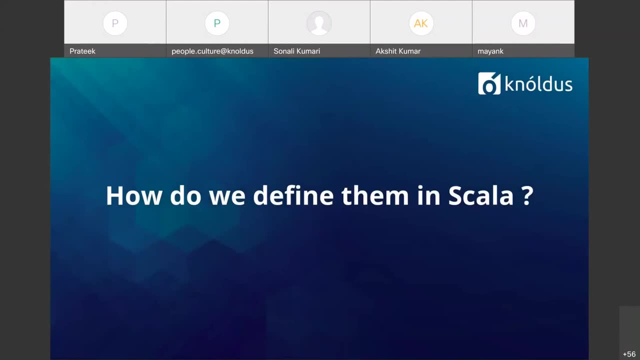 what you want, what you want to do. you don't need to specify how it will be done. so in this manner, it helps you to raise the level of abstraction. yeah, so now the question is: how do we define them in Scala? so let's see. so let's take an. 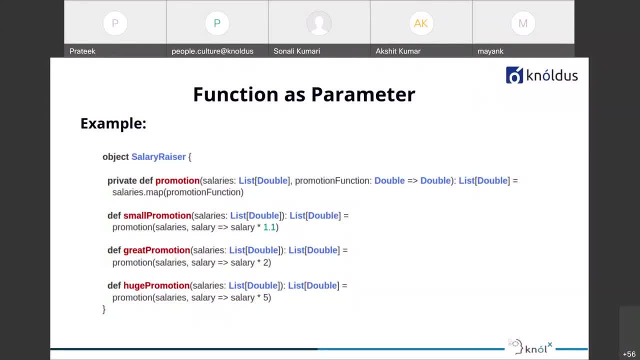 example of a high-order function that take any other function as a parameter. so here we have the salary raiser object and it contains four functions. the first one is the high-order function- how I'll explain it- and the next three are the normal functions, which is calling the higher order function. so the first 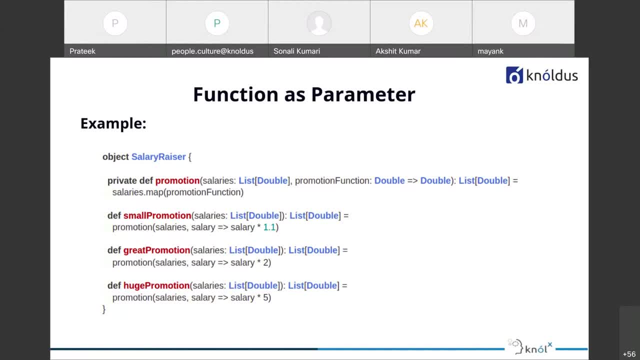 function, that is, the promotion function. it's actually a higher order functions. it has two parameters. the first one is the salaries of type list of doubles and the second one is actually a function from double to double. so the first double is actually the type of parameter that this function expects and the next double that is after the arrow. 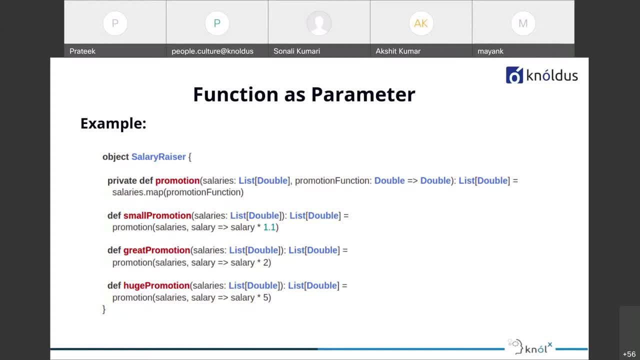 is actually the return type of this function. so here we have just we have a function that take only one parameter. that's why we have not enclosed it within the parentheses. so if we have a function that takes more than one parameter, then we can enclose that. 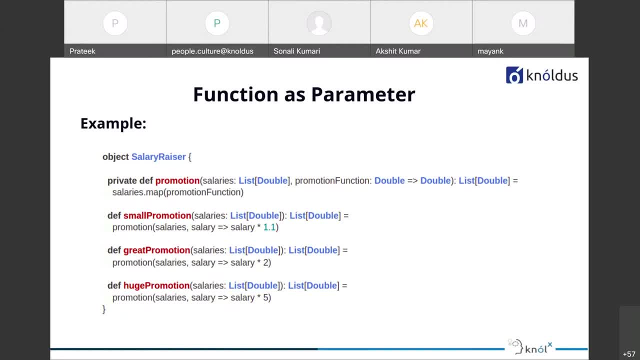 close it within the parentheses. so what we are doing here, simply the small promotion, great promotion and huge promotion. so, uh, we'll, uh, the salary will be increased based on our promotion. so if our promotion is small, then our salary will increase by uh, by some amount. so what we are doing here, simply the small function is calling the higher order function. 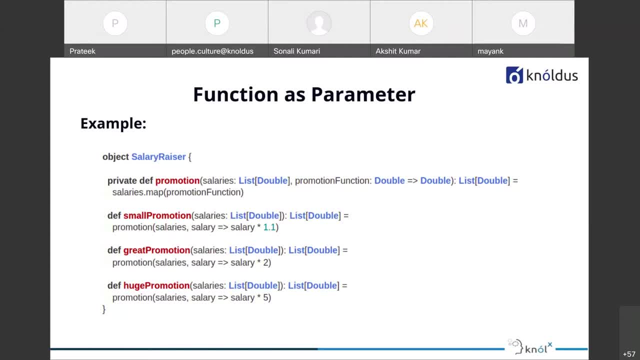 which is the promotion function, passing the salaries. and then here we are passing the body of that function. that promotion is expecting, so what we are doing- salary, and then the body salary multiplied by 1.1. so the first salary is actually the name of the very uh parameter. 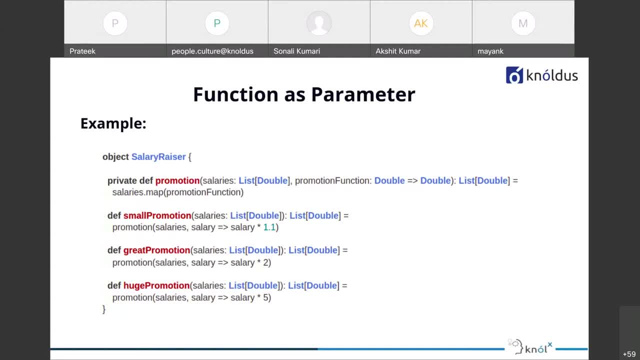 and the salary uh into 1.1 is actually the implementation of the promotion function. uh, okay, and similarly the great promotion and the huge promotion are also calling the promotion function, but they are increasing the salary uh a bit more compared to uh each other. okay, so i hope you get some idea of how we define a function that. take another function as a. 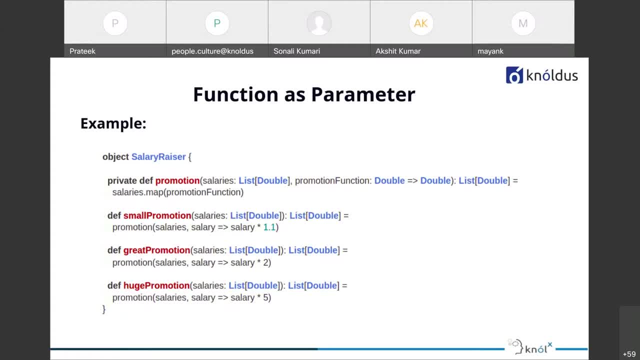 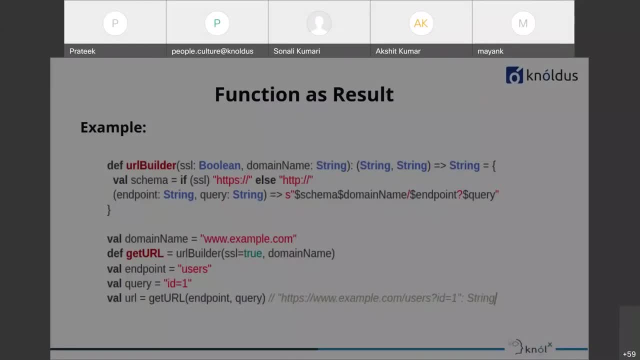 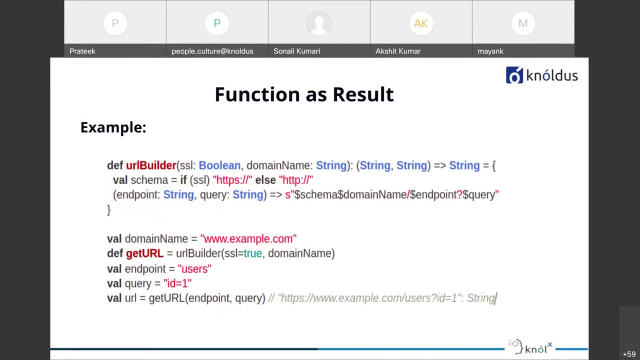 parameter, but we'll uh understand it better, uh, through the demo part. so okay, so let's see an example of a function that takes: uh sorry, that returns any function as a result. so here we have the uh url builder function that takes two parameters of type boolean. 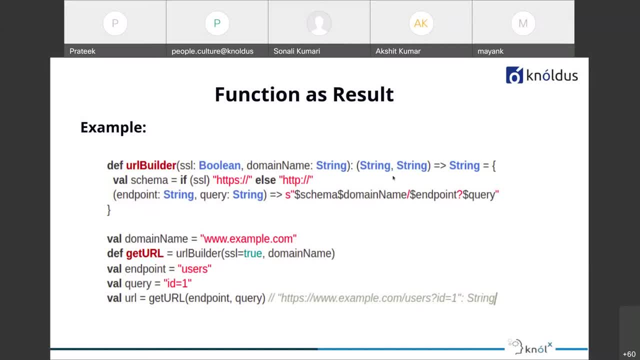 and string, and here it is returning. it is actually returning a function. so this is uh how we return uh a function from another function. so it will basically return a function that will take two parameters of type string, and the return type of that function would be, uh will be string, okay, so what we are doing here? simply we are doing. 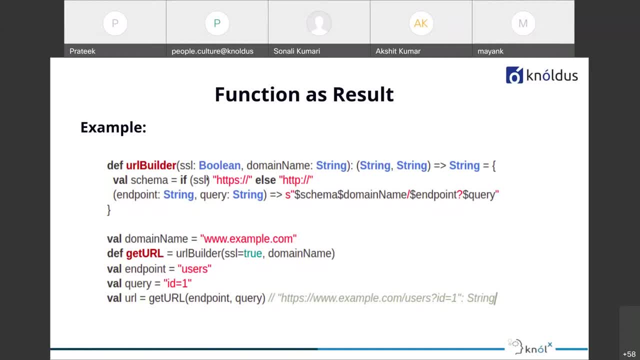 a if else here and the schema will uh uh store this string and finally, at the at this uh last line, we are returning a function, an anonymous function. an anonymous function is any function that does not have any name. so this is an anonymous function that will uh take two parameters and the return type of this function. 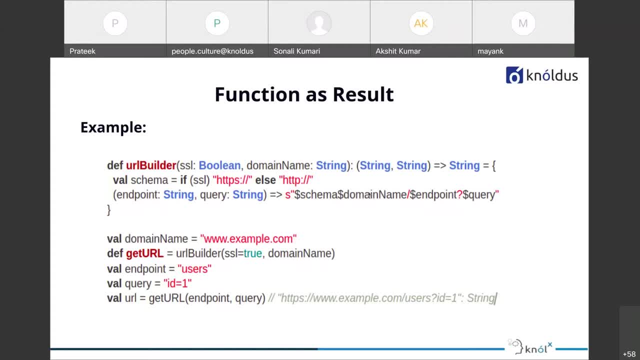 is string. so here we are actually returning a string. so this way, uh, we satisfy this uh function. okay, so how we are calling it? we are simply uh calling this url builder function and we are assigning it into the get url. so get url will be of type: uh, string, comma, string, and we are going to 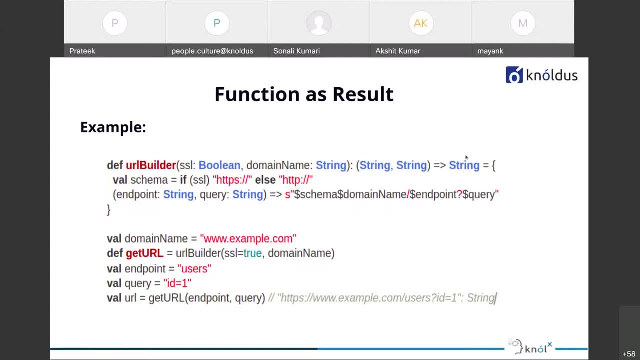 string and the return type of this function. that function will be string. So now you can see in the last line that when we are calling the get URL, we are passing the endpoint and query. both are of types string. So this way we get any function as a result. and finally, we are passing some values to. 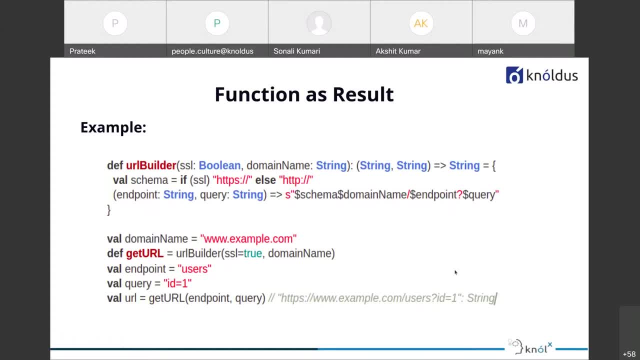 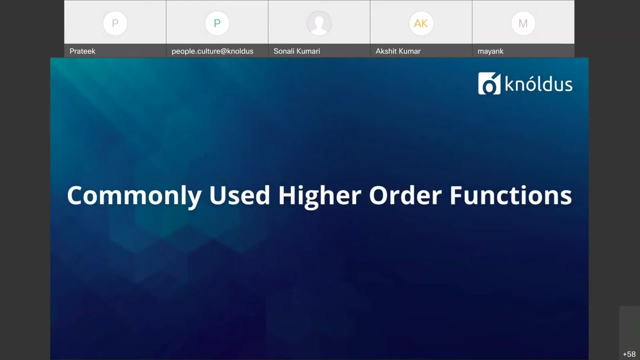 it and getting the result. So again, I will explain more about it in the implementation part. So till now, do we have any questions? Okay, let us move on to the further slide. So now we will learn about some of the common features. 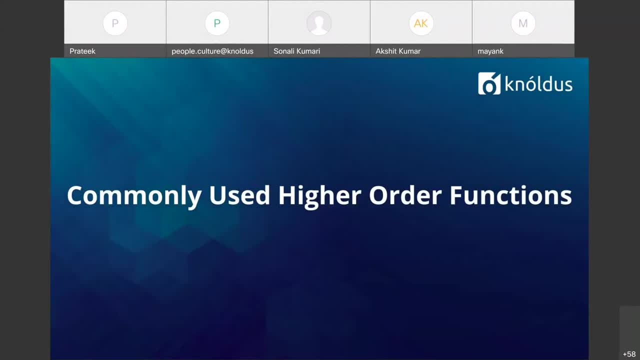 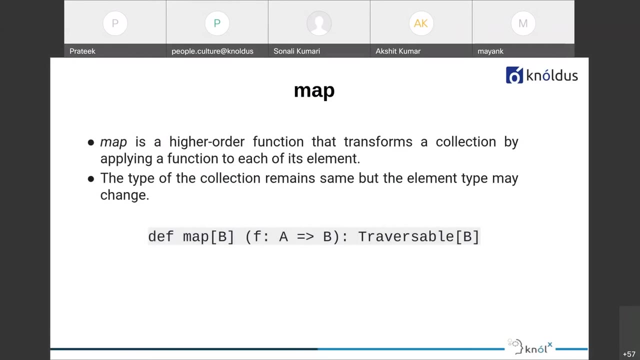 We commonly use higher-order functions in Scala. So Scala has a lot of predefined higher-order functions, and we will see some of the important ones. So first one is map. So map is simply a higher-order function that transform a collection into some other collection. 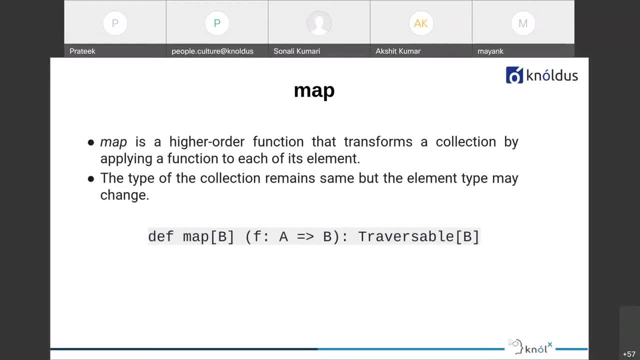 by applying a function to each of its elements. Okay, So one point to note here is that the type of the collection remains same, but the element type may change. So here we can see how a map function looks like. So it basically expects a function from a to b. 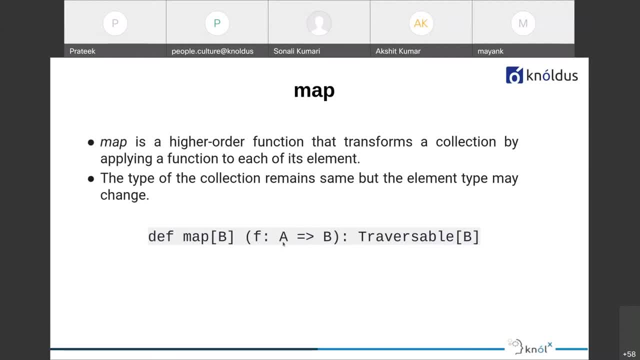 So a to b in the sense means a function with only one parameter And it returns. It returns us a traversable which is the top-level class in the hierarchy of collection, in the collection hierarchy. So this is how the map signature looks like. 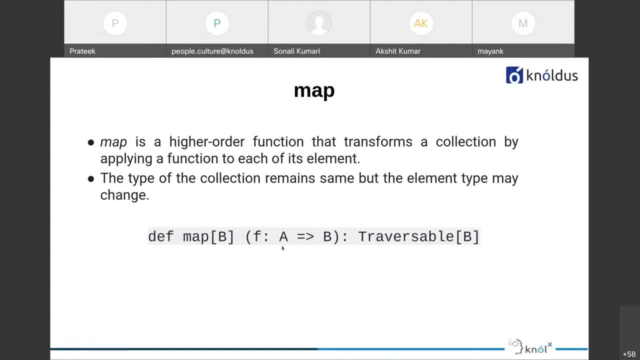 So this map function will call this function that we have passed here- the f on each of the elements of the collection- and will transform it based on the implementation that we will provide, And this is how it works. So the next important higher-order function is flatMap. 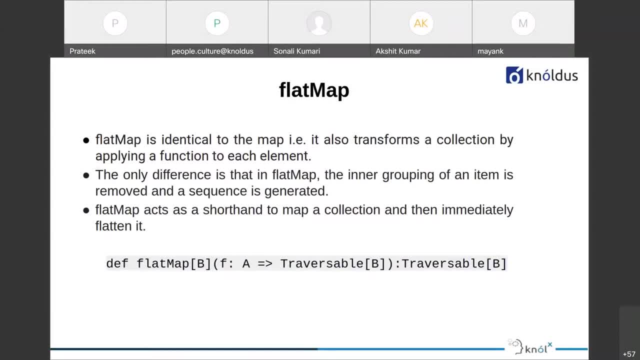 So flatMap is identical to the map function, So it also transforms a collection into another collection by applying a function to each of its elements. But what's the difference? So the only difference between map and flatMap is that in flatMap the function is a little. 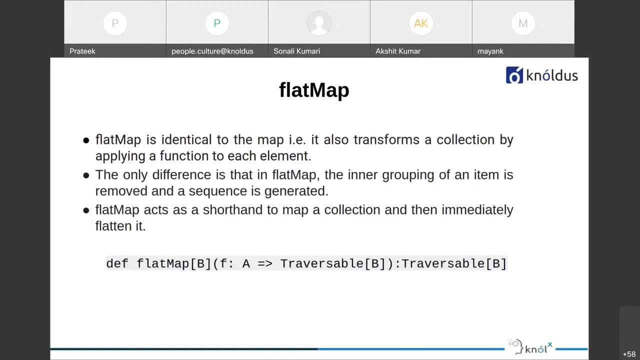 smaller. In flat map the inner grouping grouping of the elements are removed and the sequence is generated. So let's say, if you have a list of list of integers, then when we call the flat map function on that and it will convert the list of list of integers into a 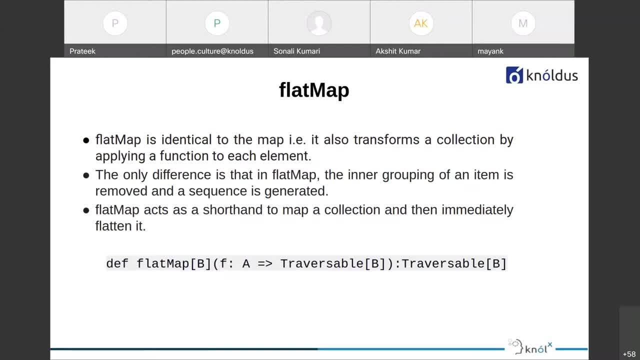 single list of integers. So what it has done? it simply removes the inner grouping of the elements and generate a sequence. So flat map acts as a sort and to map a collection and then immediately flatten it. so in other, in simple word, we can say that Calling prep flat map is 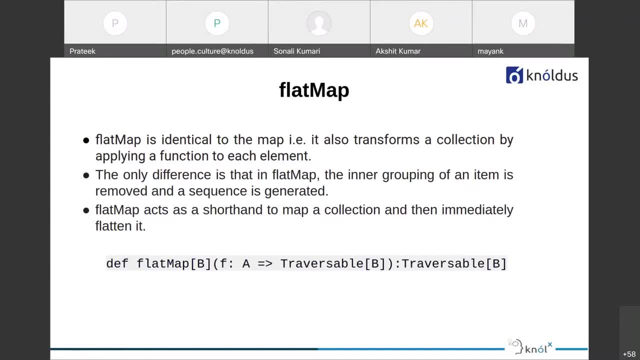 Like calling the map function, followed by the flatten function. so We'll also see how it works in the Demo part. so this is how The signature of flat map looks like. so it expects a function from a to traversable of B. so, as we have mentioned, 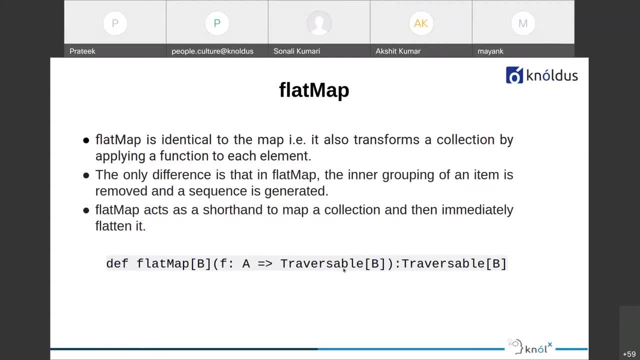 it will return us a collection and The inner grouping of that collection will be removed and finally we'll get the. We get a single collection of some type. Okay, so this was all about flat map, so Let's move on to the other. I order function filter. so. 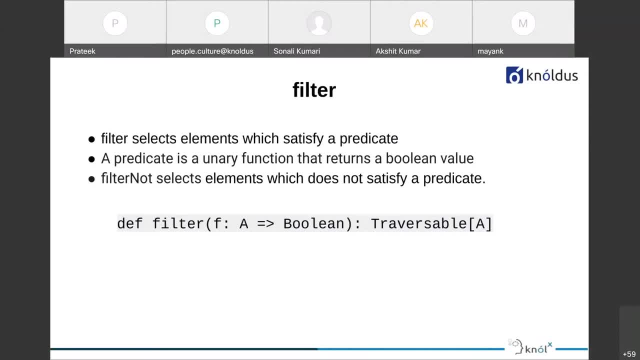 Filter basically removes the unwanted data from the collection. or we can say: filter select those elements would satisfy a predicate. So what's a predicate? So a predicate is nothing but a unary function that returns a Boolean value. So here in the signature of this filter function, you can see: 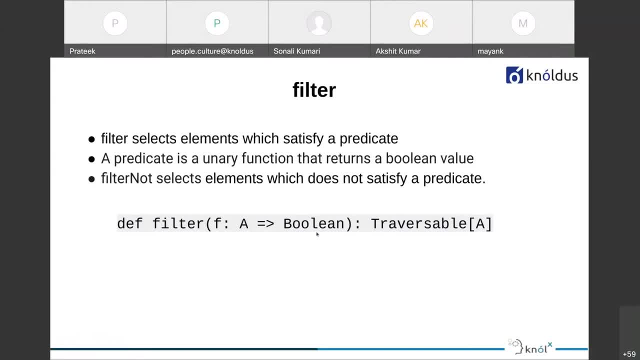 This Filter is expecting a function from a to Boolean. It's actually the predicate or the unary function having only one parameter. so it will Call this predicate on each of the element of the collection and if this predicate or the condition satisfy for that element, then it will append it in the 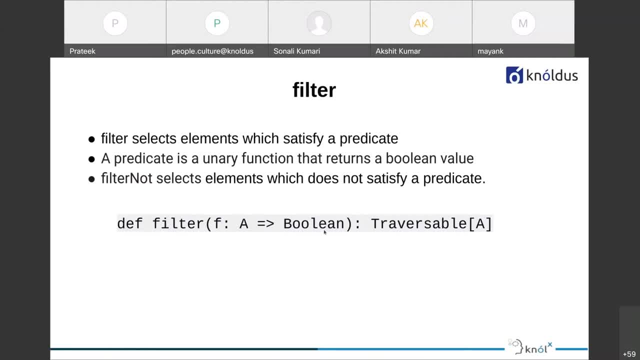 resultant list or the any type of collection that we'll have. so we Also have filter not, which is, which is just the opposite of filter. So filter, not select elements based, which does not satisfy a predicate. so this was All about the filter function. so let's. 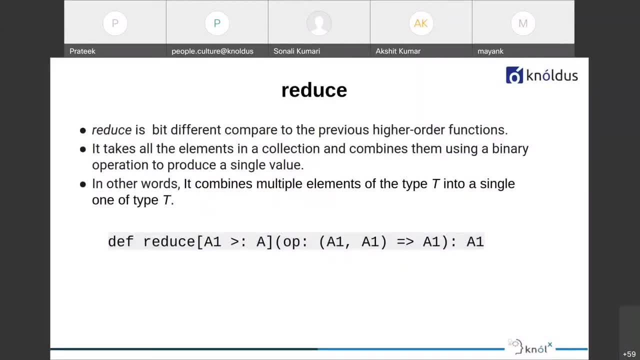 move on to the next one. this is reduce. so Reduce is a bit different function function compared to the previous one: the map, the flat map and the filter function. How it is different, let's understand that. So reduce function simply takes all the elements from a collection and combine them using a. 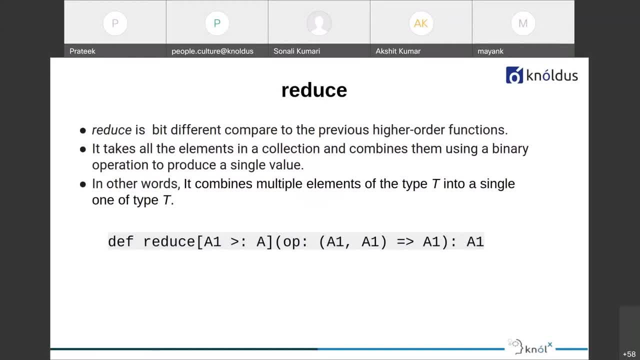 binary operation to produce a single value. So if we are calling the reduce function on a list of, let's say, double, then it will combine all the doubles and will return us a single element of the same type that is double. So you can see that, in other words, it combines multiple elements of type T into a single. 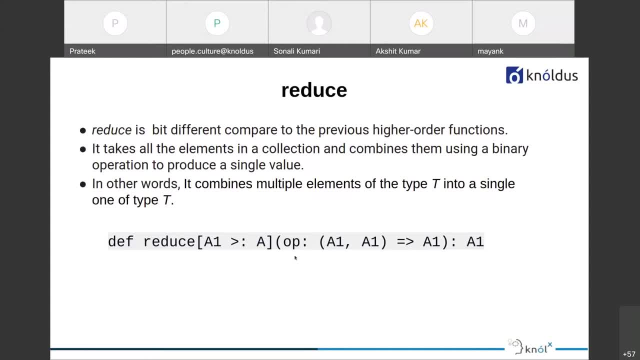 one of type T. So here we can see. this reduce function is actually expecting a binary operation or a function with two parameters and return a result, And it will call this function on each of them. So this is how reduce is different from the other ones. 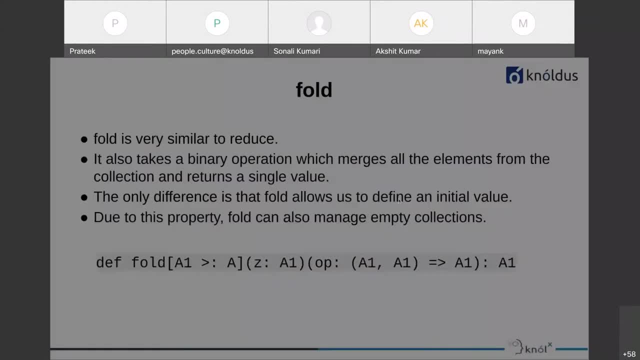 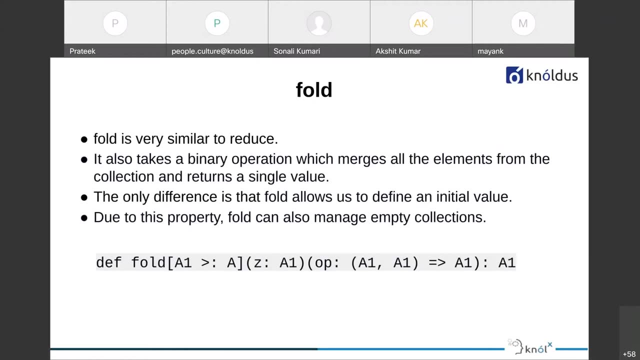 So let's move on to the final higher order function, which is the fold. So fold is quite similar to reduce, So it also takes a binary function. So it takes a binary function. So it takes a binary function Which merges all the elements from the collection and returns a single value. 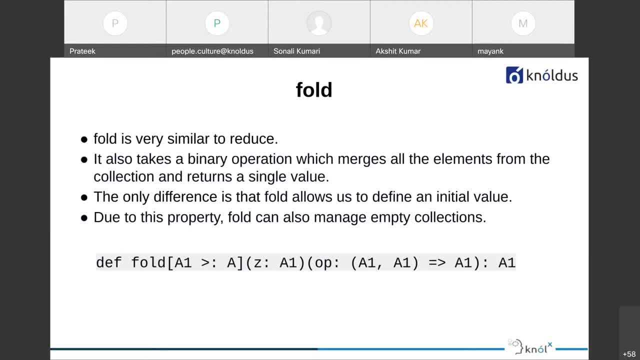 So in this bin, fold is similar to reduce, But there is a difference. The difference between the reduce and the fold function is that fold allows us to define an initial value for the accumulator, So what that accumulator is. So accumulator is nothing but a variable that keeps, that is responsible for keeping the 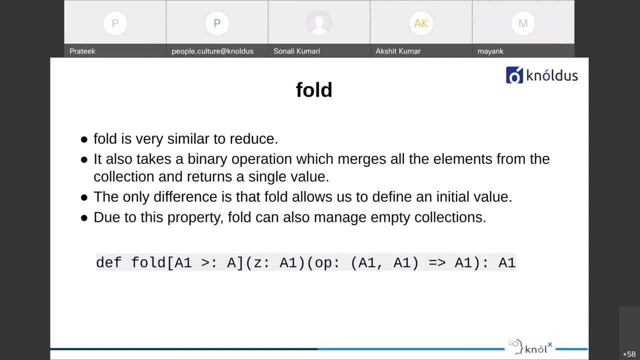 that are performed on that collection. we'll also understand about it in the implementation of: okay, so, uh, due to this property, fold can also manage empty collection. okay so uh, how uh that works? so in case of reduce, we don't have the concept of initial value, but here we have the concept of initial value. so, uh, in case of, uh, any empty. 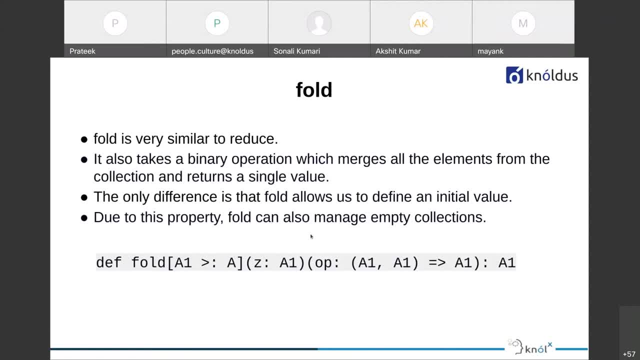 collection. so fold will basically return this initial value as a result of that function. but in case of reduce we don't have any initial value. so, uh, we'll get some kind of exception or unsupported operation exception, such kind of- i'm not sure about the exact exception, but 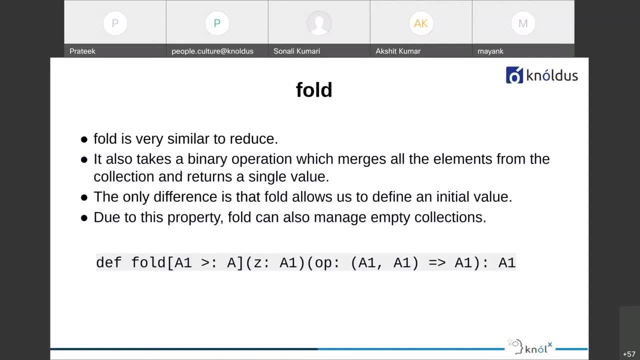 we cannot use reduce on empty collection, but fold can be used on empty collection. similarly, here is the signature of fold. so this z colon a1 is actually, uh, the first parameter, which is the initial for any for the initial value, and the second one is same as the reduce. 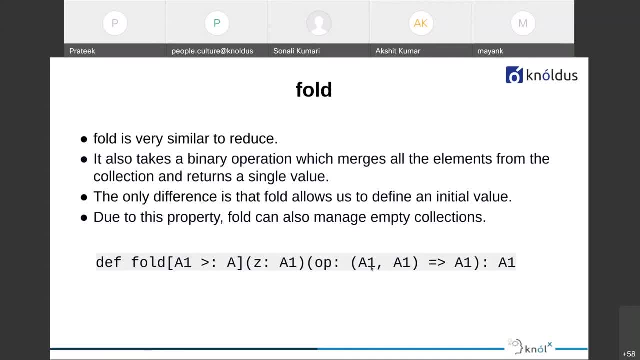 function, which is actually the binary operation, and here we'll pass, uh, our two arguments and we'll perform some computation on that, and finally it will also return us a single element. so, uh, till now, do we have any question? um, after that we'll move on to the demo part. 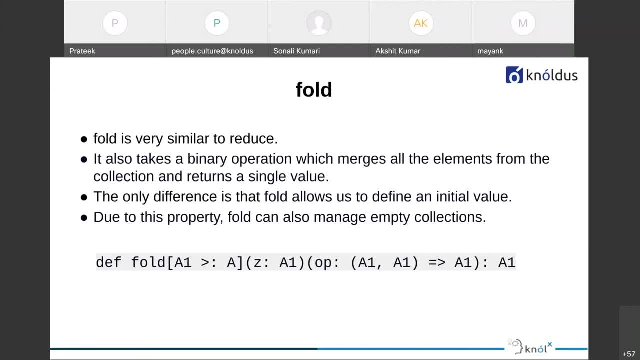 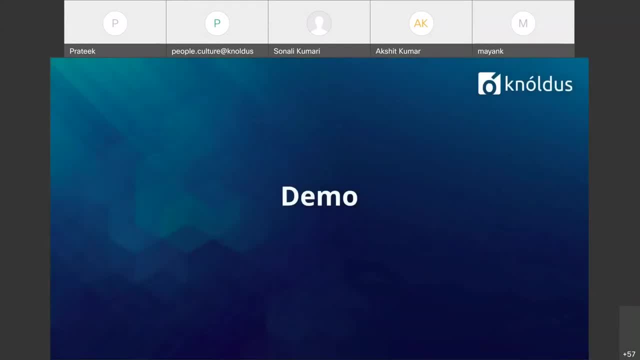 anyone. hello, am i audible? you are audible, okay. so, yes, yes, i just ask you to guys: if you have any question on query, you can ask prateek, else prateek will continue his session. prateek, i think, uh, you should proceed, okay. okay, cool, so let's move on towards the demo part. so 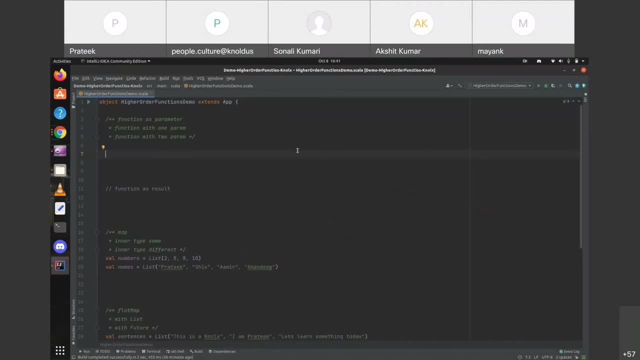 uh, we have this simple uh high order function, this singleton object, and we'll perform all the uh high order functions here. so let's take an example of a high order function. that take any function as a parameter. so simply, let's say we have a function, let's call it higher functions. 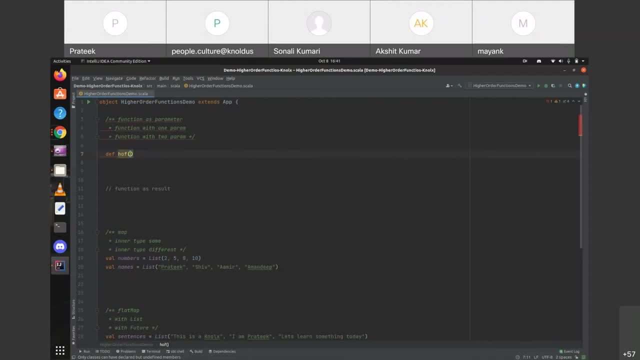 in short, then we have a function that is a parameter, we have a number. it's a num of type int and basically takes a function from, let's say, integer, and it will also return us. so what we are doing, we are simply calling this function in the body of this function. 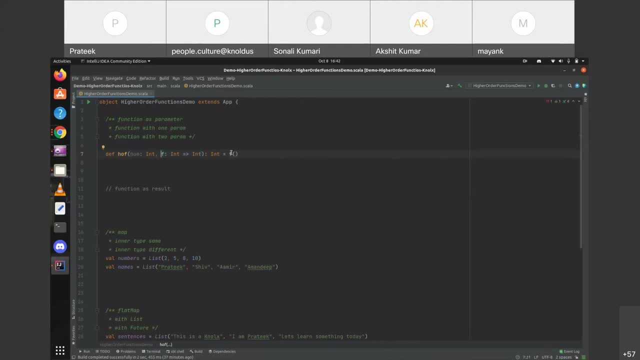 so whatever the user will pass here, that function will be called on this number. okay, so here we are simply defining a function from integer to integer. so this integer is actually the parameter of that function and this is the return type. okay, so let's see how we can call it. so we'll simply call this function. we'll pass the first. 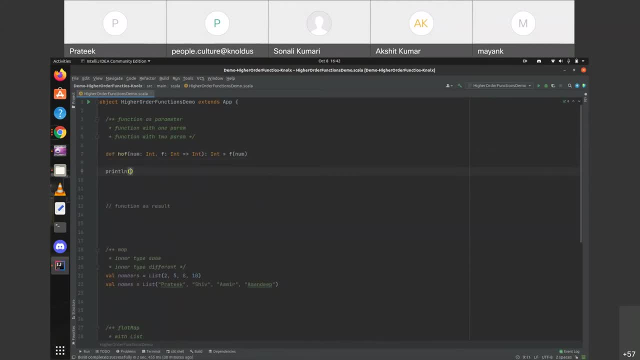 let's call it, so we'll pass the first parameter. let's say five and okay, so we'll pass the body of this, uh, integer to integer this function. so let's say so. here what we are doing. we are simply saying that, whatever that the number is passed here, just increase that number by one, so hopefully we'll get. 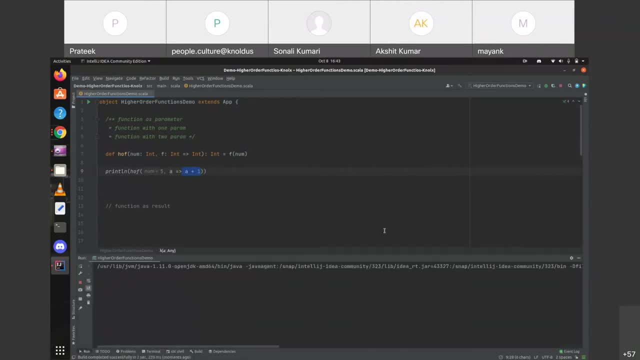 uh 6 as the output. so you can see similarly: uh, if we want to pass some other function, let's say, uh, we want uh to multiply it by two, then we will simply change the implementation here and then it will work. 10 is the output, as we are expecting. so let's take one other uh, other example. 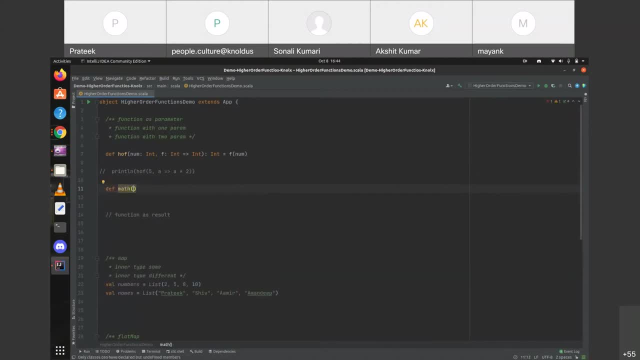 let's say this is the map function and it takes two numbers. and third is the function parameter. uh, let's say we are calling it arithmetic operation and what we are doing here? we are simply defining a function that can take two parameters and return as a result of the same type. 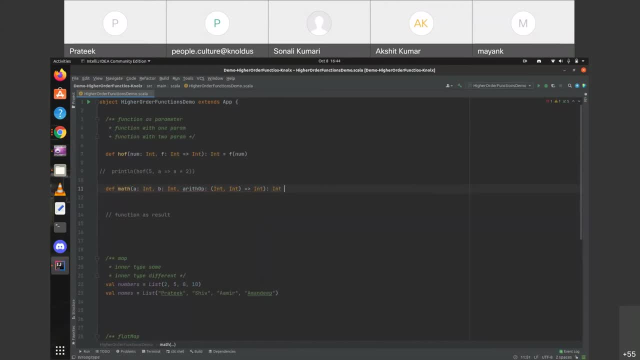 and to pass the type of this function as well, and then we will call this automatic operation and after that we'll pass the values. here they're gonna be these: uh, these two values. so we have simply defined a function, uh, that will take two uh parameters of type int and uh, and the automatic operation of 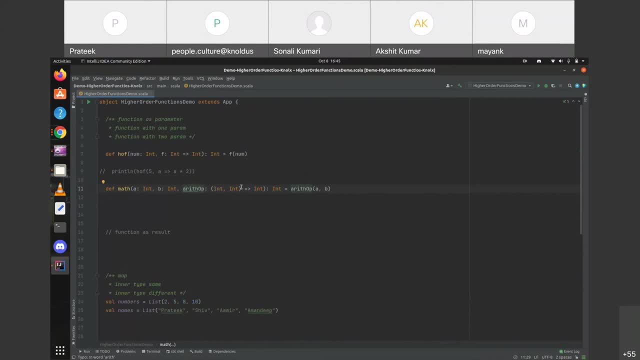 for uh type int, comma int, which is the parameters, and the return type of that function is eight. okay, so let's see how we can call it. let's say first one is five, second one is: that's the first one is uh 15, the second one is: 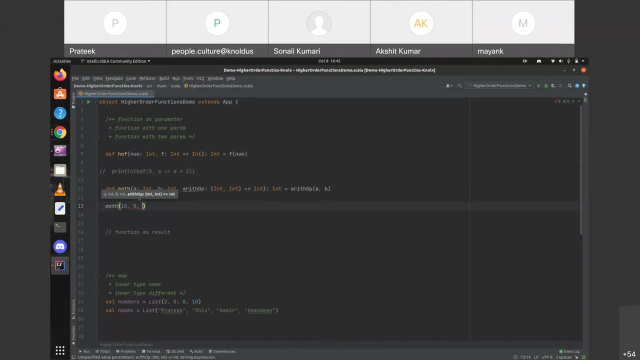 um eight. and then now let's say we want to perform the addition operation, then we'll simply do it like this: uh a comma b, then we'll return the addition of those two numbers. so this is how we'll perform the addition operation, and let's print it. 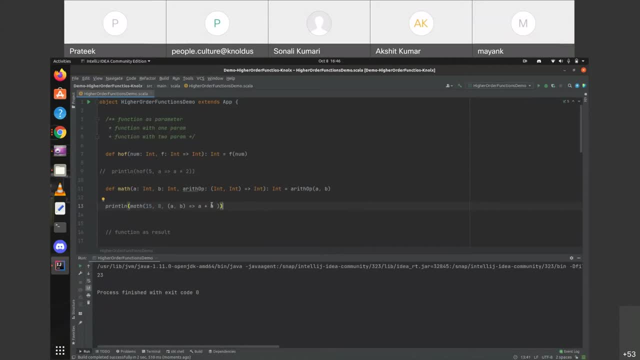 so see uh here. uh, it is returning as the uh addition of these two numbers. so how it is actually working: it is simply taking the implementation from here and calling the same function on these two parameters. so, similarly, if we want to perform subtraction, then we can simply do it like this: 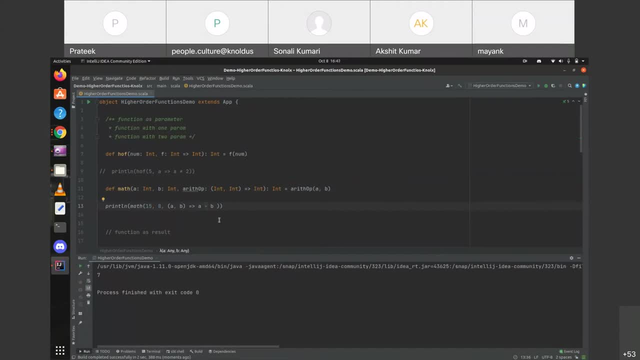 it will actually take some as an argument. this is actually an anonymous function, that is, a function without a name. so we can also do it with some other way. let's say, we define a add function that will take an, that will take two- uh parameters, something let's see. 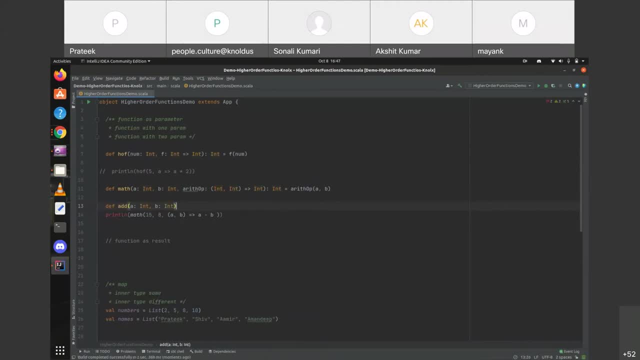 so let's take two and it will return us write a plus b. similarly, we can also have the subtract function. that will return us the subtraction of this. so instead of defining the function here, we can simply pass the function of the same signature. let's say add, without the parenthesis. 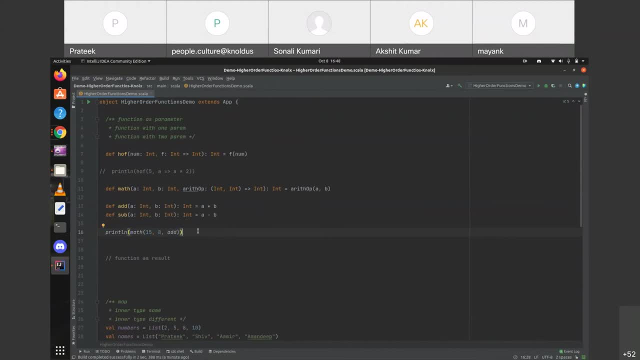 so it will work the same way like the previous one. so if we call the, we will get the output as 23. similarly, if we pass- if we pass- subtract function without the parenthesis, then it will give us the subtraction 7. ok, so this was all about the function. 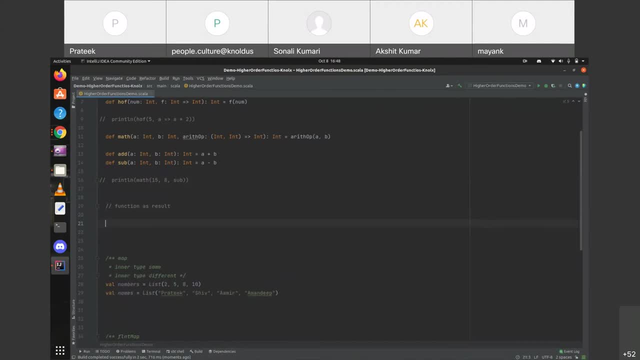 as parameter. now we will see some example of function. as a result, we will use the same math function, but in a different way. so let's say math2, and it's simply taking the operation name as a string and it will return us a function. so here we are defining. 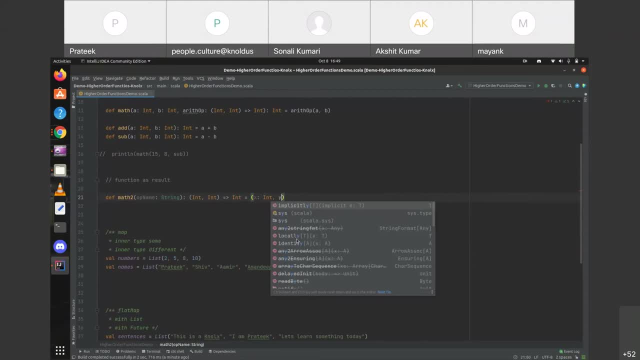 parameters of the function that will be returned based on the operation name. it will return the function as so we are calling the match there. so if it's a add function, then simply return the addition. so if it's a 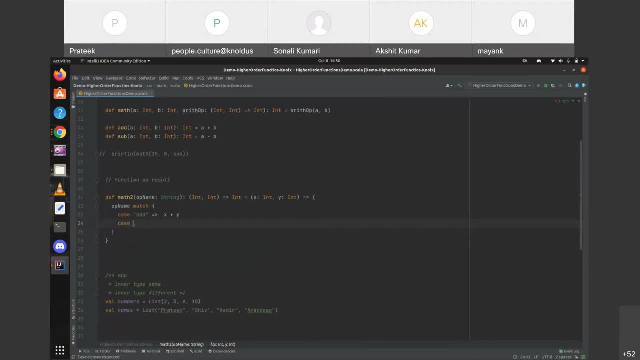 subtraction operation, then it will return us the subtraction. so how it is actually working. it is actually. it is taking the operation name as a string and based on that it will match uh, that string, uh, with these cases and. 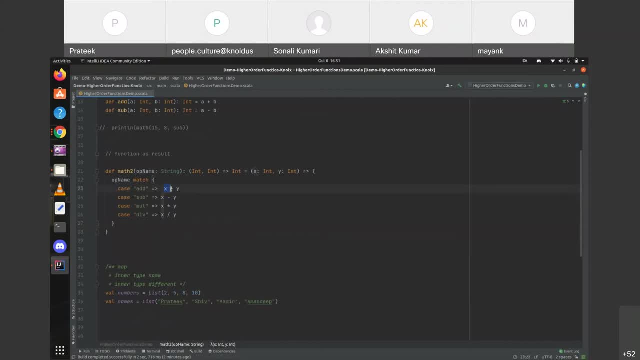 whatever the operation name will be, then it will return the implementation based on that. so let's uh use this function. well, let's say we want uh to perform addition function. we'll call the math to function, we'll pass, add in it and let's see what it returns us. 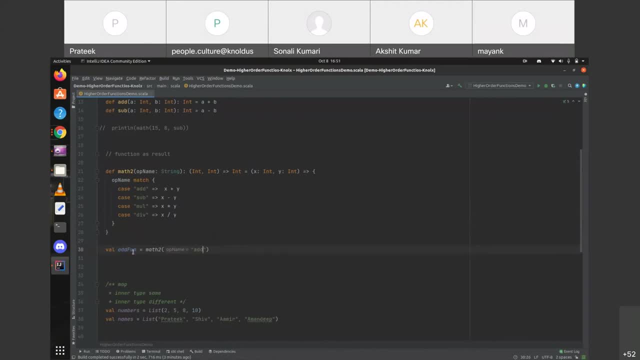 see it's returning us a function. that's so. it's returning us a function, uh, that will take two parameters and will return us a integer. similarly, like this, it's actually returning the same function. so similarly for, let's say, subtraction correction, then it will also return us the same function. but now how we call that. 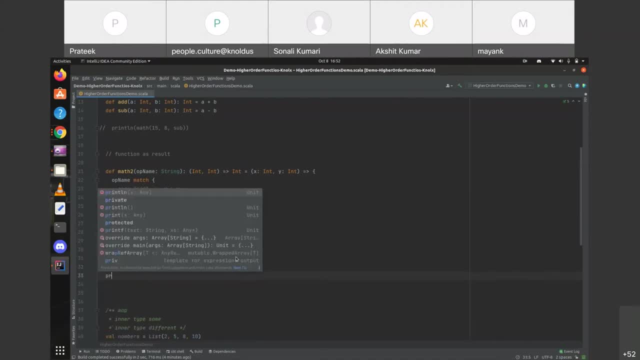 call these add and subtraction function. so simply, we'll call this add function. we'll pass the parameters in it, let's say five comma eight, and similarly uh. for the subtraction function. let's say we are calling the subtraction function with two parameters: 20, nine. let's see what we'll get. 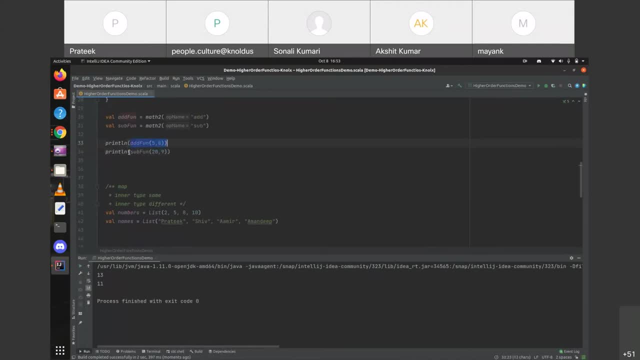 see, it's simply returning us the addition and this one is returning as the subtraction. and similarly, we can also, uh, define the multiplication function and the division function. it's uh, that will also work the same way. so this was all about the function as a result. okay, so now we'll see. 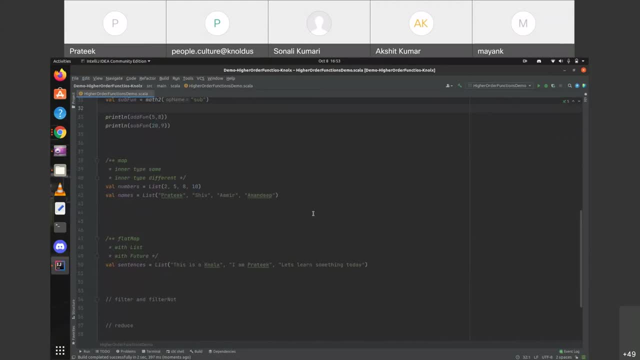 some of the uh commonly used higher order function, uh in loose. so simply first let me comment out. so let's use the map function first. so here we have simply a list of numbers, integers and the list of string, so let's call the map function on each of them. let's see. 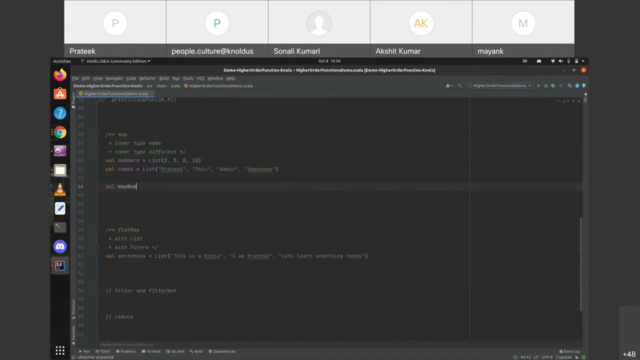 others, just like saying: well, map, numbers, dot, map, and what we'll do? we'll simply increment each of the number by one. so you can see, here it's returning us a list of integers. uh, and let's paint this and see what we have from here. what's the output? so see, this function will be called on each of these elements. 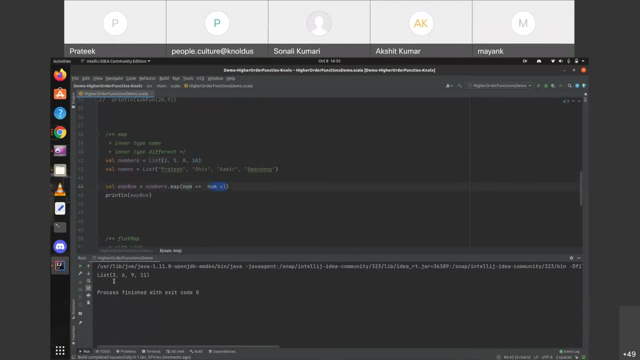 and it will increment them by one, and that's why we are getting three, six, nine and eleven as the output. so one other way or the uh shorthand for the calling the same function would be uh. instead of passing the whole function, we can simply do it like this: underscore plus. 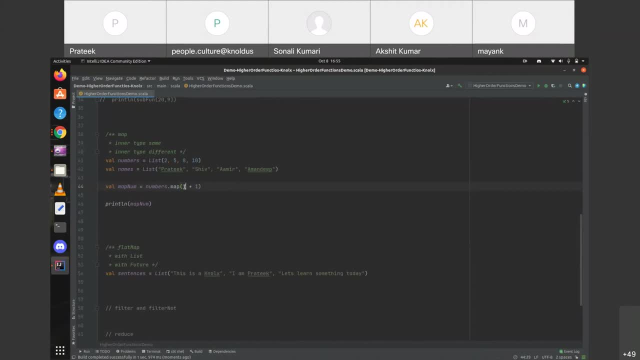 one, it will also give us the same result. so this underscore represent one function parameter, or we can say this underscore will represent each of this element. okay, so again, let's check the output. so we'll get the same output. so it's an example of calling the map function. that will return us. 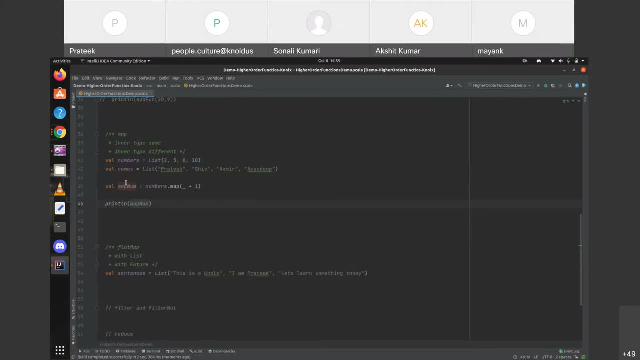 the same type. so, as we have discussed in this slide, that the outer type, which is list, will remain same, but the inner type, that is, these elements that may change. so in this case we are getting list of integers because we are returning the 진행. 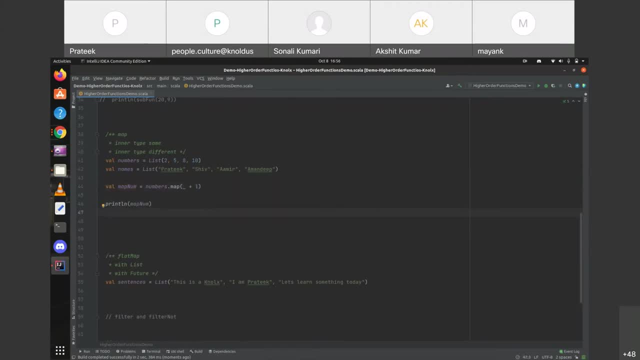 integers. but let's take an example where the inner element type will be will be changed. so let's say map names. so what we are doing, simply names, dot, map, and what we'll do? we'll simply take each of the name and we'll return the length. so this: 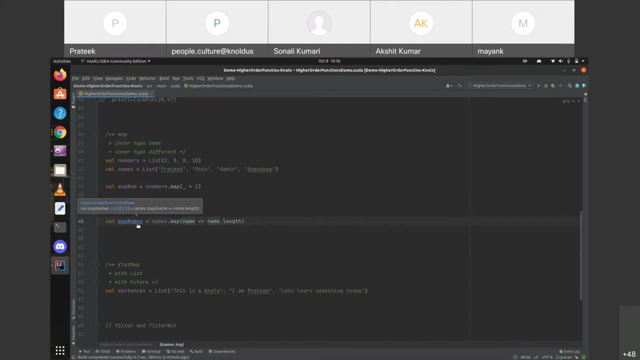 way, if we check the type of this map names, we can see it is returning us the list of integers, but it's actually the list of string. but on calling the map function, it's written as the list of integers. because of this, you change the type of inner element here, so this function will be called on each of. 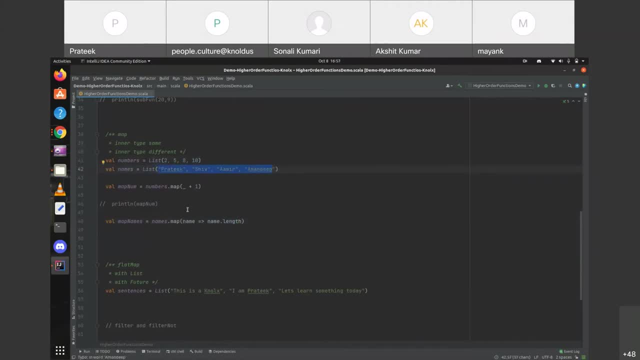 these names and it will return us the length and this way, the inner type will be changed. let's check it. so we are getting the length of each of these strings. so this is something that we were 3 what. this is something that we were expecting. similarly, we can also do it like this: 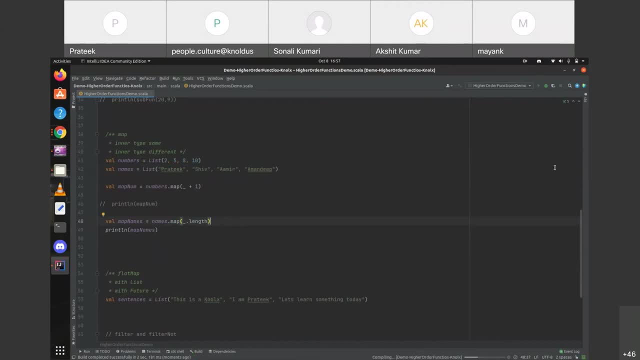 it was the same either. okay, so now let's move on to the other. okay, so now let's move on to the other part. now let's see the flat map. some examples of flat map. so we have sentences and we simply have a list of integers. now we'll quickly see an example of flat map. 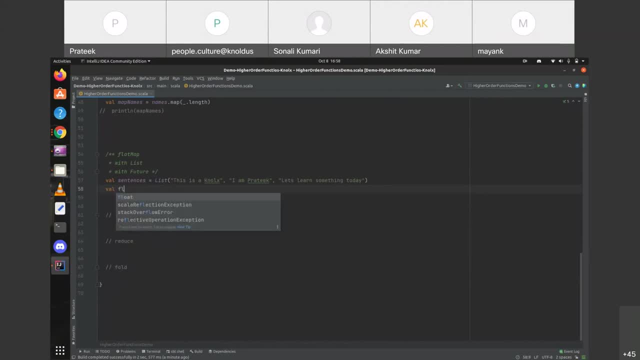 you can give it any other name. so sentences dot. let's say first we try to call map on it, so map and simply what we are doing the sentence okay. so we are taking each of the string and we are splitting in uh into uh, its words and what we are getting here. we are getting a list of 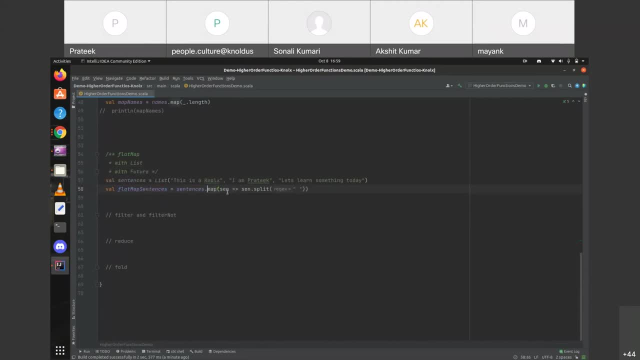 array of string, but instead of calling map, if we call flat map here, then it will convert it into a list of integers. that is, uh, it removes the inner grouping and generated a single list of. generated a single sequence. so we can print this out: flat map sentences. 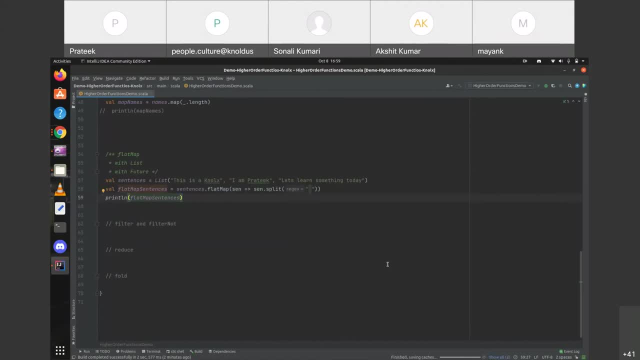 see array just like a list. that's why so, as i mentioned in the slide, that calling flat map is like calling the map function, followed by flatten. it will give us the same result. see this. so if i hover on it then it will say: replace dot map and flat. uh, flatten with. 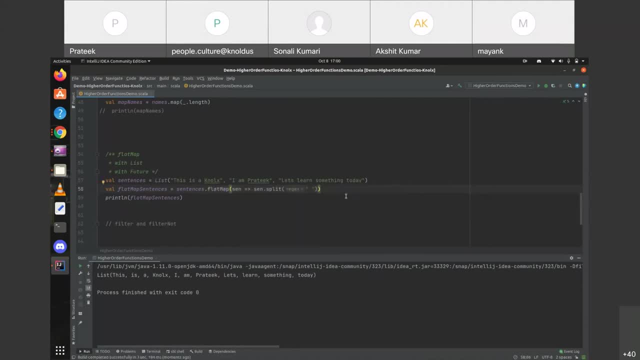 flat map. it's the same uh as calling map and the flatten function. so this was, uh, an example of using the flat. we can. we can also use it on futures. let's say, if we have a future of future of, let's say, int, then the flat map function will convert that future of future. 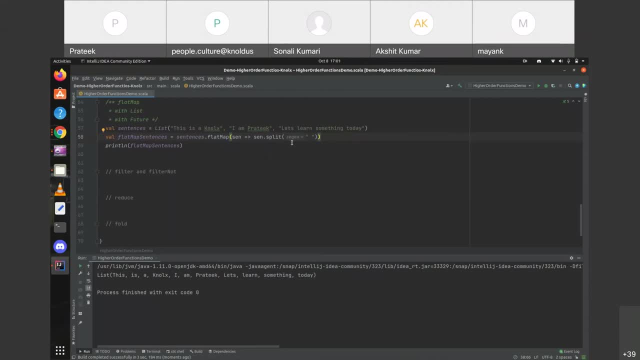 of int into a single future of it. not just that, if we have a future of future of int, then also it will convert it into a single future of it. so this was an example of flat map. let's quickly see the example of filter. so let's use this uh number list here as well. 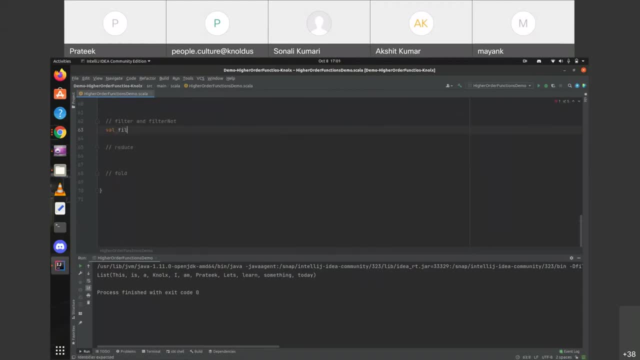 so well, equals to numbersfilter and we'll simply pass the condition here. let's say n and n should be greater than five. then let's print the output. so see um. the num list of numbers is containing two, five, eight and ten, but two and five is. 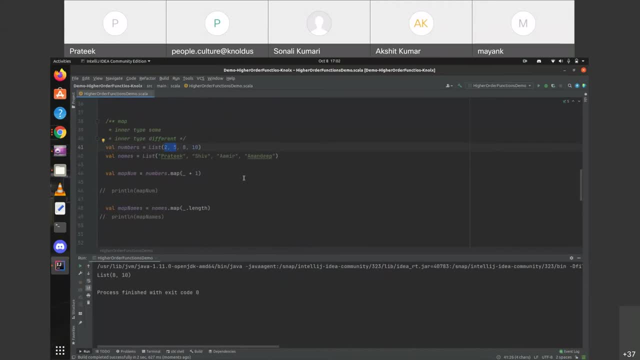 not satisfying the predicate. that's why it's not added in the list. but eight and five is uh satisfying that predicate. that's why we get eight and ten uh as the output of this filter function. similarly, we can use filter not here and that will work. oppose it, so let's. 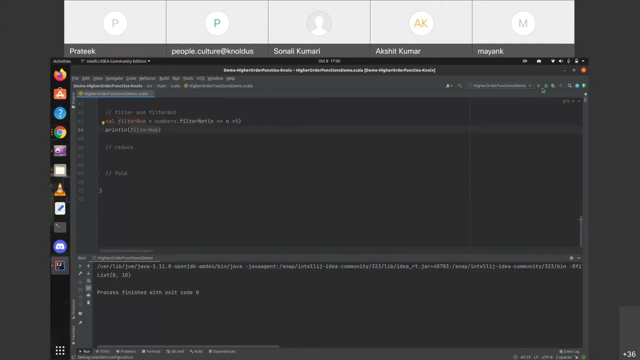 use filter, not here, and that will work. oppose it. so let's use filter, not here, and that will work. oppose it to filter, to filter. now we'll get list of two and five. see, this is the output here. so as uh, let's quickly see the examples of reduce and fold as well. so they are quite similar. 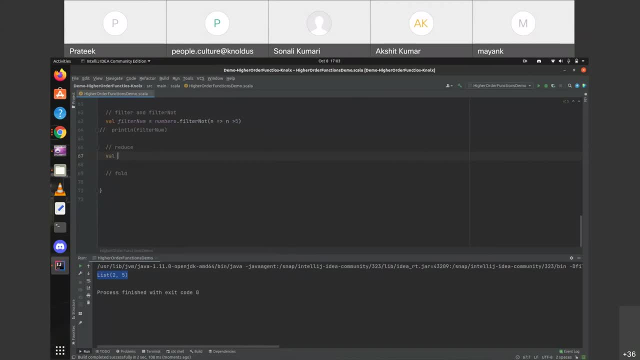 so, well, well, we are using the same numbers, list we are calling, which is of, list of, in which is of type, list of integers, reduce. then we are simply, uh, passing the binary operation here, and what we are doing? so, uh, we can see that. so, uh, we can see that. 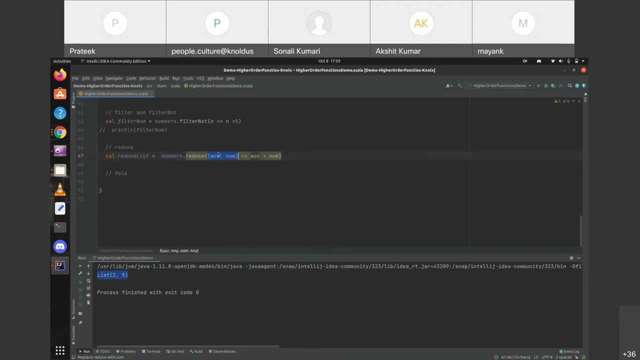 so, uh, we can see that we are passing the two uh parameters here. we are passing the two uh parameters here. we are passing the two uh parameters here. first one is the accumulator. we are first. one is the accumulator, we are first. one is the accumulator. we are simply giving name to those. 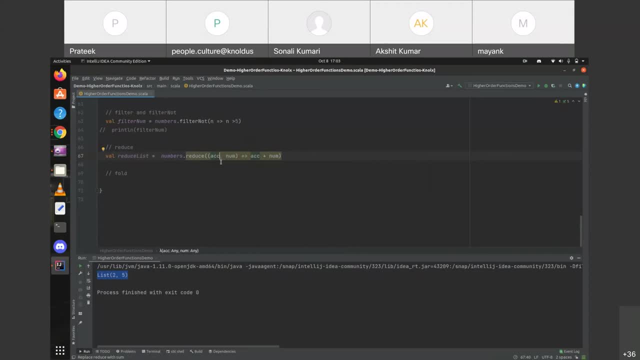 simply giving name to those, simply giving name to those types: accumulator, basically types. accumulator, basically types. accumulator basically accumulates, or keep the state of all accumulates, or keep the state of all accumulates, or keep the state of all the calculation, the calculation, the calculation and and. 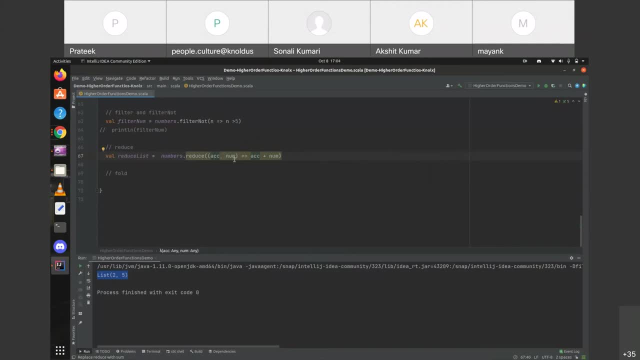 and finally we'll be, we'll get the output. finally we'll be. we'll get the output, finally we'll be. we'll get the output from the accumulator, from the accumulator, from the accumulator. so if we print the output here, so if we print the output here, 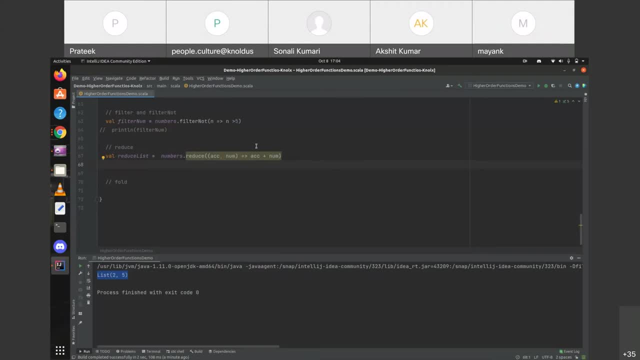 so we are simply taking every element and adding it with the next one. so bin lm reduce list: see the addition of all these elements is 25. that's why we are getting us. so you can see that it's returning us an integer, just an int, and it's a list of int. so it's converting a list of int in. 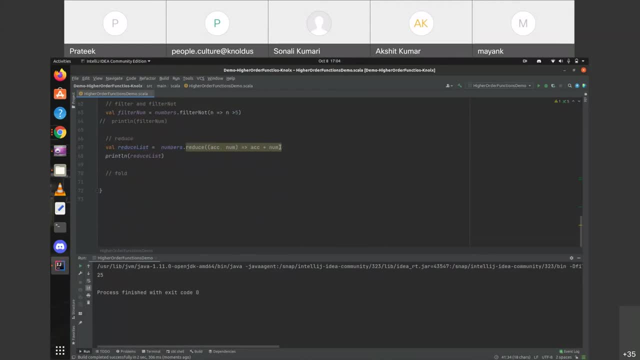 just a single element of type of the same type. okay. so here we are doing the sum. we can also perform some other operation, like that's multiplication, so it will give us the multiplication of all the numbers, see, okay. so finally, let's see the example of the fold function. 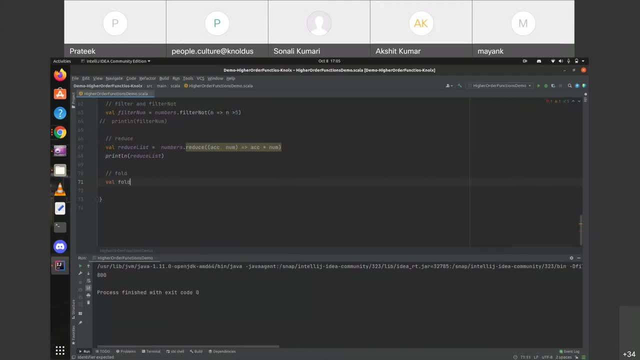 so we can give an example how to use that. so, as we have discussed, the difference between reduce and hold is we can pass an initial value to fold, so let's pass 0 as the initial value. otherwise, if we don't pass the initial value, uh, in this reduction function, because we don't have that option, so it will take. 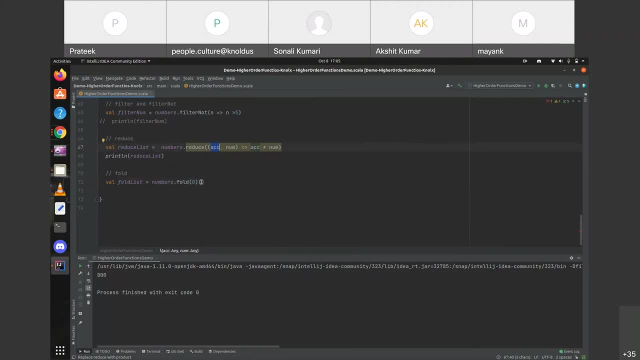 the first element as the initial value for this accumulator. so similarly, we'll pass a binary operation here and plus number. so see, uh, this will also give us the same output. so actually there we are doing the addition. uh, let's say, if we want to uh change the initialized value, then we can simply do it. then this uh over this highlighted: 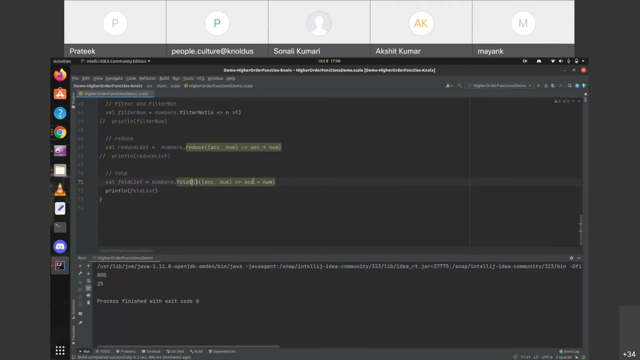 error will be gone. initially it was showing us that we can use some instead of calling this whole, because here at that time we were simply adding all the elements. but let's say we change the initial value value, then it that will be gone. so the in this case the initial value is 35 and the 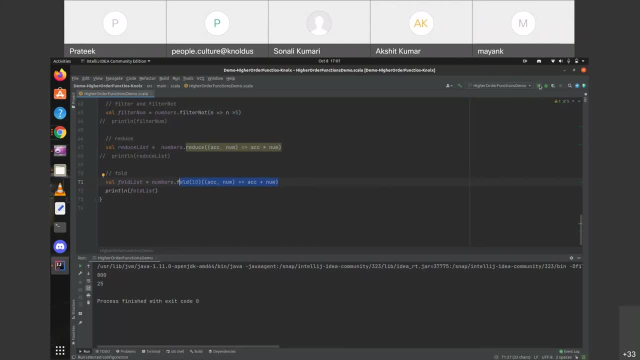 sum of all that elements will be 25, so we'll get 35 as the output, because we change the initial value. see, 35 is the output. so, as i discussed, uh, in case of reduce, we cannot uh reduce with an empty list. so, uh, if let's say we remove all the elements here, so this will 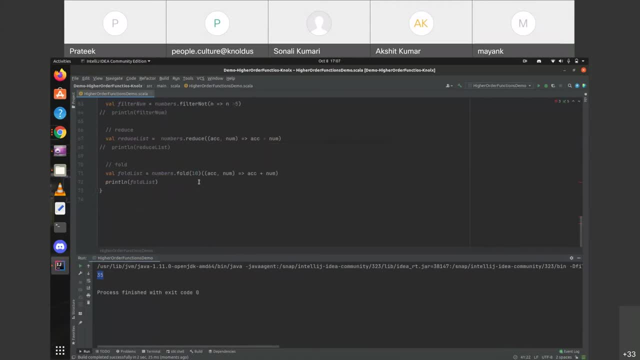 give us an error, but this will not give us any area, so let's quickly comment out all these. so now, in this case, we have an empty list, which means this is because we need to remove the list as prime as possible. so the next step is to remove first the sample cell, so um use. 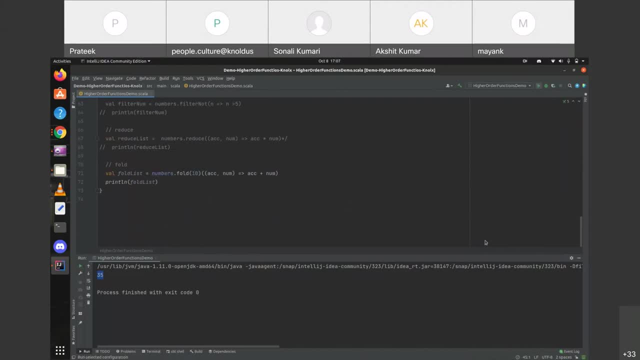 empty list. so in this case, let's see the output. so, as i told you, it will take this initial value as the output of this whole list, whole operation, if we have a empty list. so this was all about the high order functions. so if you, if anyone, has any question, then they. 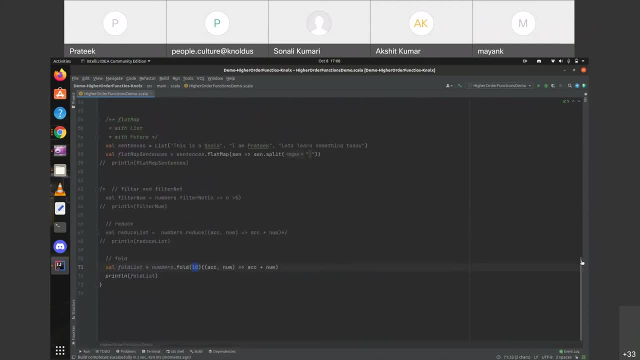 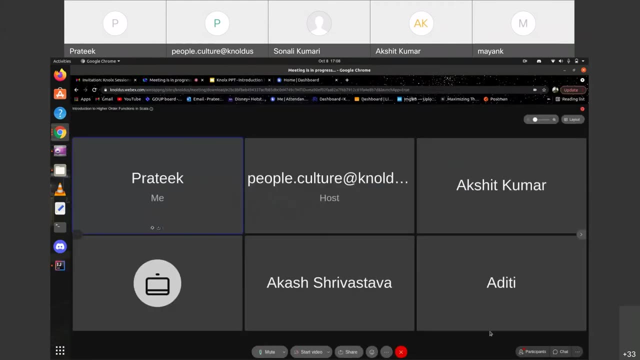 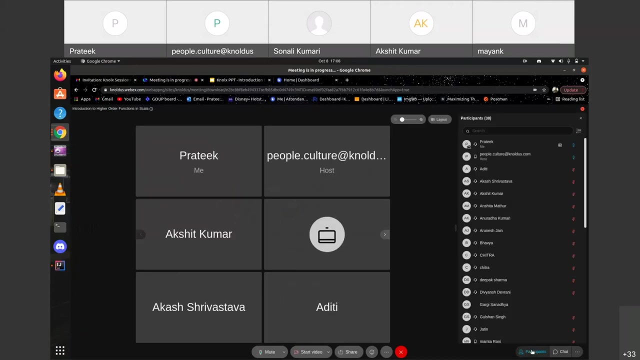 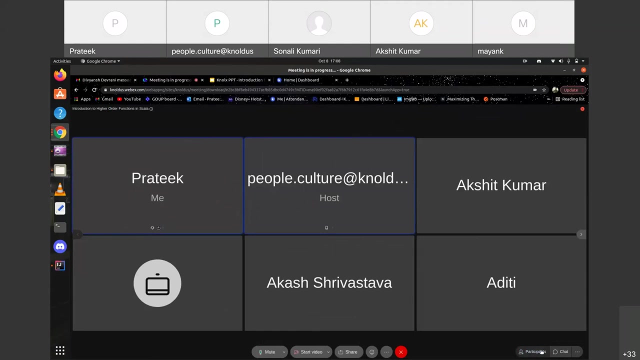 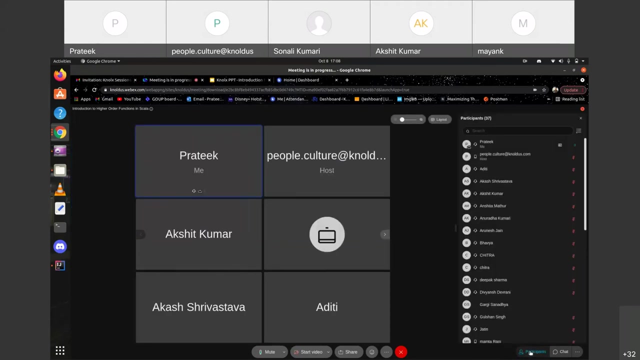 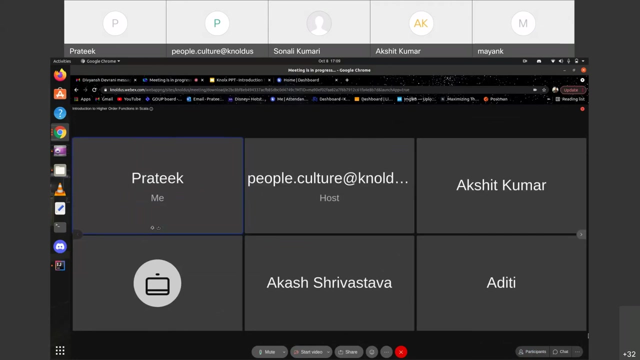 can ask. so do we have any questions? guys, if you have any question, you may ask. it will help the facilitator to understand that. you know, uh, on which thing he has to reiterate, so we all will be glad to know. i think, uh, they don't have any question. if you have something to share, more, you can. 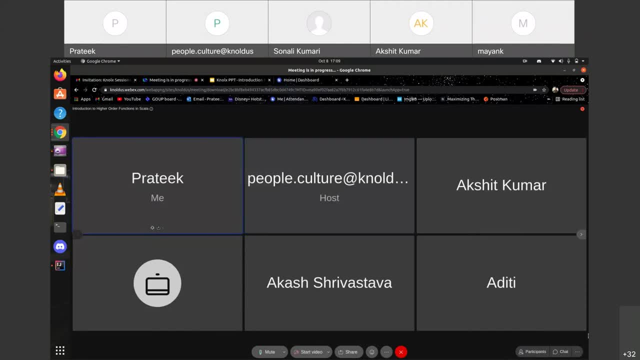 so, no problem, it was uh uh. hopefully, uh, you will understand something uh new in this session. uh, i think it was a easy session for everyone and yeah uh. so please, uh uh submit a feedback for this session so that if there is something uh that i missed, then i will definitely try to. 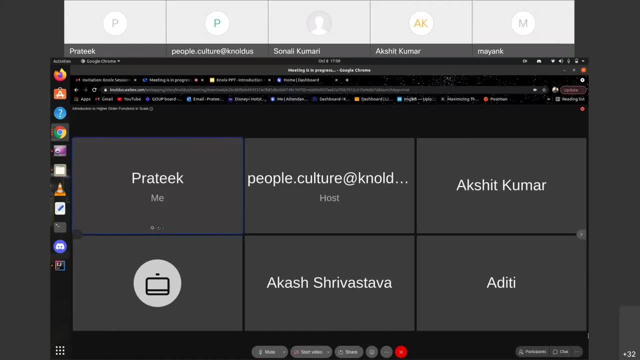 improve that the next session. so, yeah, thank you so much everyone. thank you, prateek, for this wonderful session. uh, however, i am, i'm amazed that there are 40 people, and who are not even, you know, considering to unmute themselves and share their thoughts on, uh, this, so this. 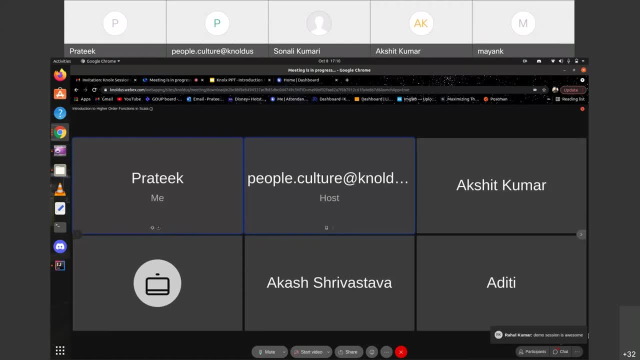 is? uh, you know, this is a surprise thing to know. uh, rahul, we all would appreciate if you can, you know. uh, i would like to thank you for this wonderful session and i hope you will unmute yourself and let us know that how you felt about the session- even everyone. 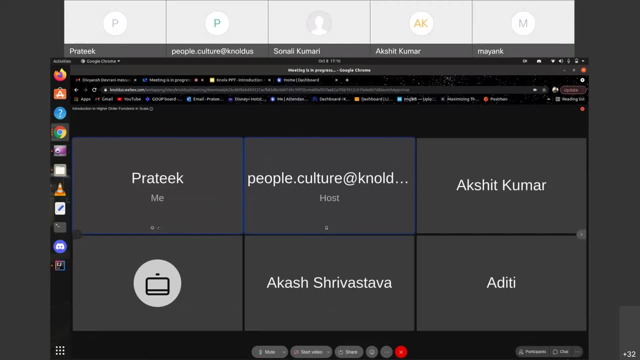 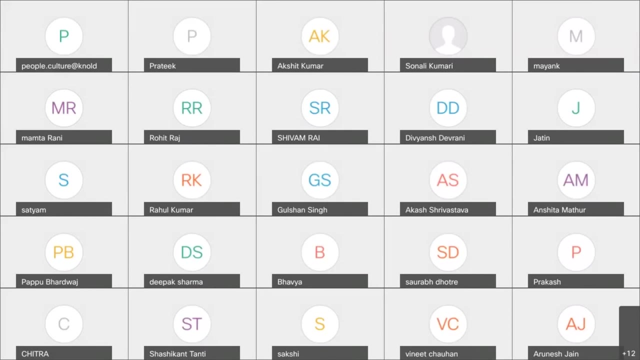 who is reacting, who are all are giving reactions. we do appreciate, but, uh, it would be highly appreciable if you all can unmute yourself and let us know about the session. yeah, yeah, yeah, yeah, yeah, yeah, yeah. thank you so much everyone. thank you for taking out time and attending this beautiful 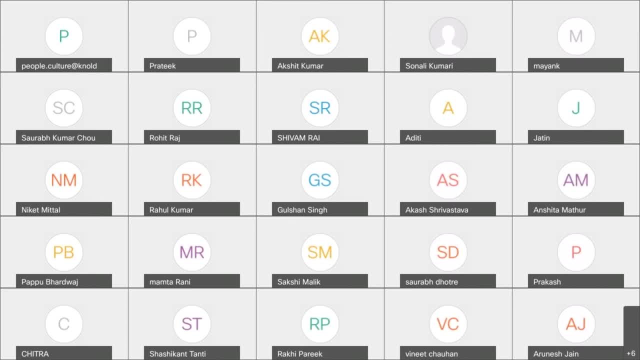 session by prateek and prateek. i really, really appreciate your time and efforts for this. so, uh, let let's share our feedback and feedback forms and let the facilitator know, uh, you know what are the things which you know he or anyone else needs to. you know the previous. 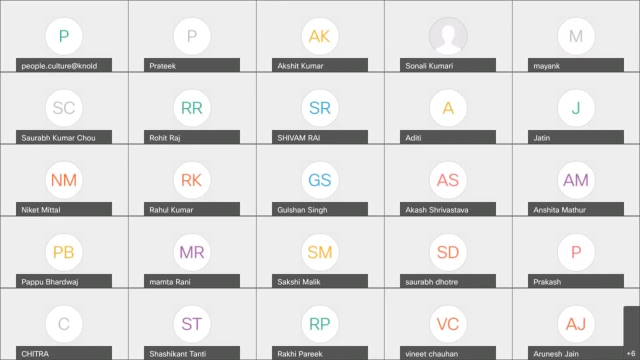 session also needs to cover. so, uh, we are waiting for your constructive feedback. thank you, guys. thank you so much. once again, welcome.